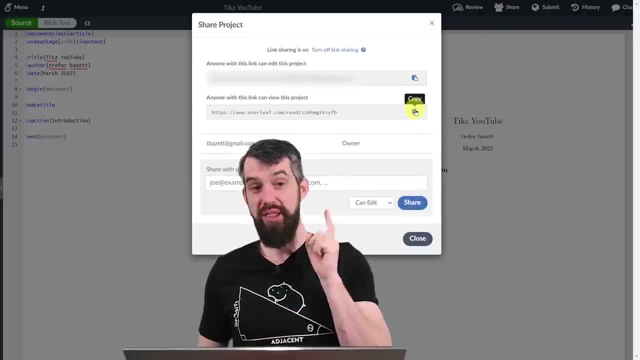 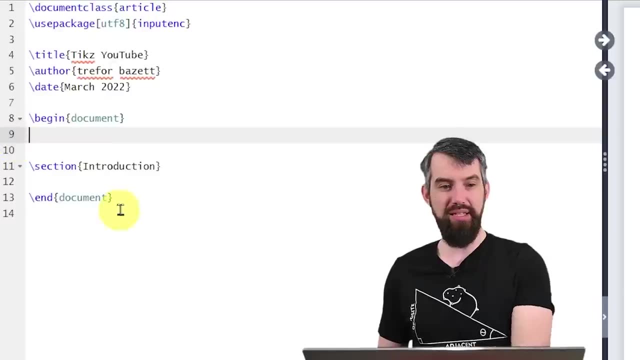 document, And so I am going to share this link. That link will be down in the description. It's just a really nice feature of Overleaf. Now I don't actually need a title page, so I will get rid of this, And this little bit of code is what we begin with in a so-called blank document. Now, 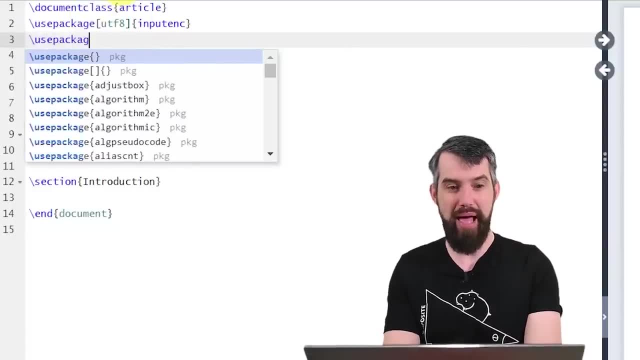 I want to use Tixi, so I'm going to add this package using Tixi. So I'm going to add this package using Tixi. So I'm going to add this package- use package- and I'm going to add Tixi, and I'm actually going to add one more. It's going to 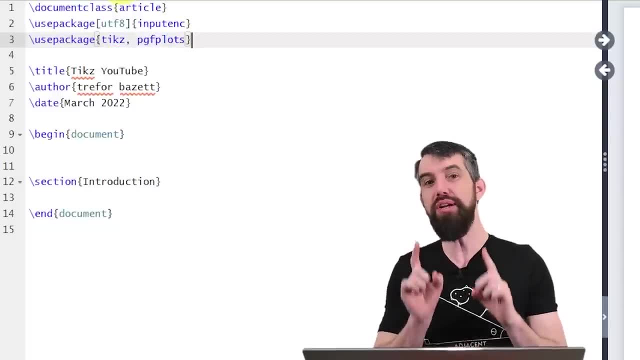 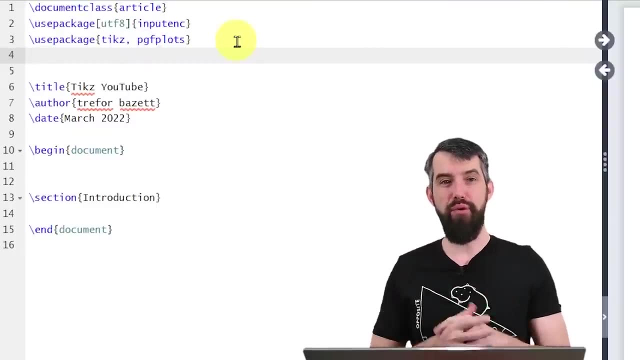 be called pgfplots. These are two different packages that we're going to use in tandem. a little bit for this video. There's one other thing that I'm going to add in this preamble before I get going. I'm going to say: use tix library, and then I'm going to add something called. 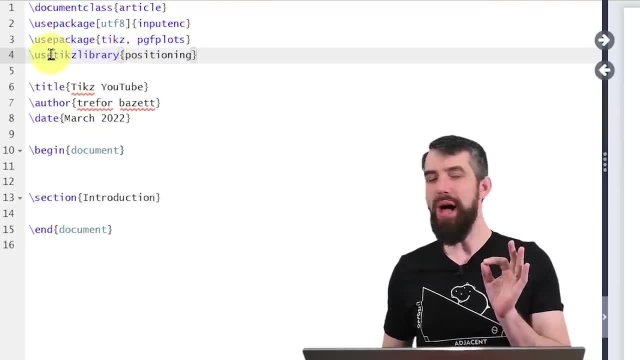 positioning And basically there's a whole bunch of different extra libraries that you can add that give ever expanded functionality on the core tix package, And I'm only going to use one of those, but there's many of them that you can use. That is now my preamble, Okay, so let's actually get. 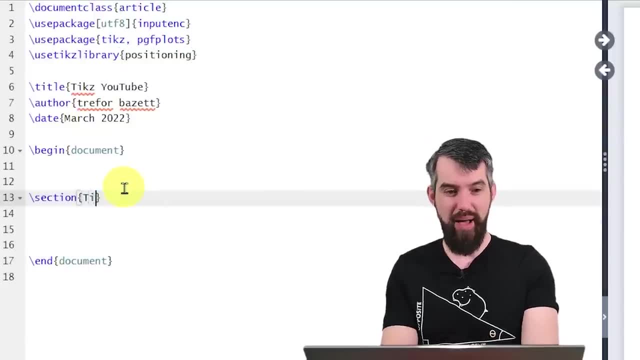 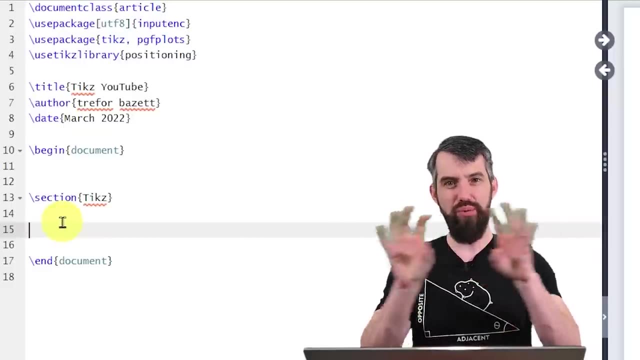 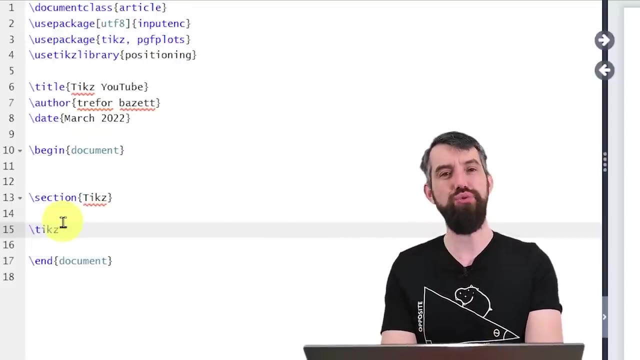 going here. I'm going to change the title of my section to Tixi, and now I'm going to do my very first thing. So if I want to make just a single graphic that's only got one item to it, I can start it by writing backslash: Tixi. And in this case I want to draw. how about some lines? So I'm going to 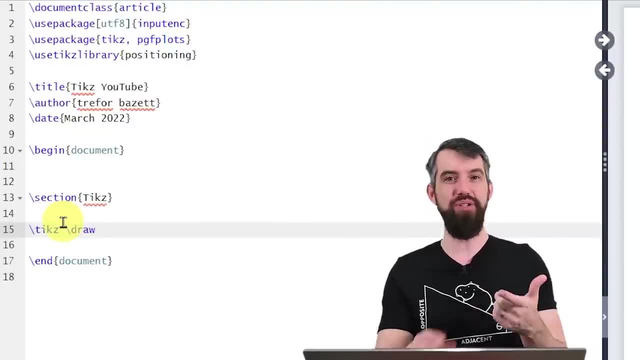 go backslash tixi, And then I'm going to go backslash tixi, And then I'm going to go backslash draw And draw. lets me draw many different things, And I'm specifically going to. how about I do this? 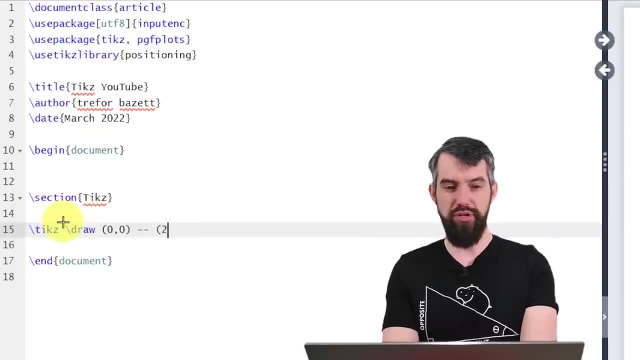 I'm going to do a line that starts at zero, zero, goes over to- I don't know- the point 2- 1, and then goes over to I don't know how, about the point 3, 2, something like that Semicolon at the end, And I'm 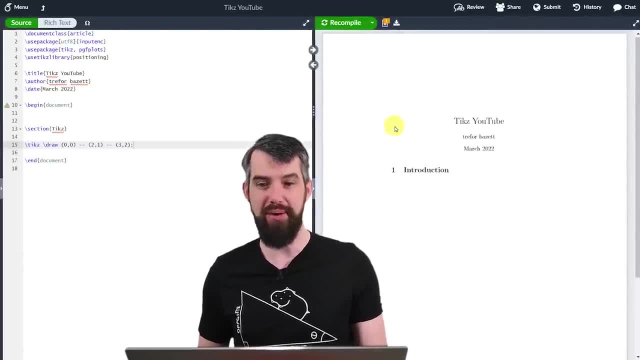 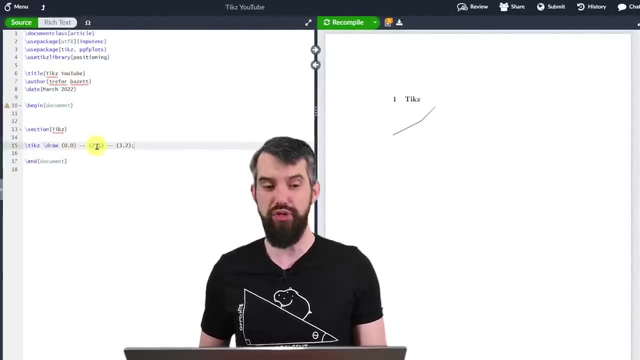 going to come and click the recompile button to visualize what it is that I get. And this is what I have. It is a pair of line segments connected, one from 0: 0 to 2: 1 and another one from 2: 1 to 3: 2.. 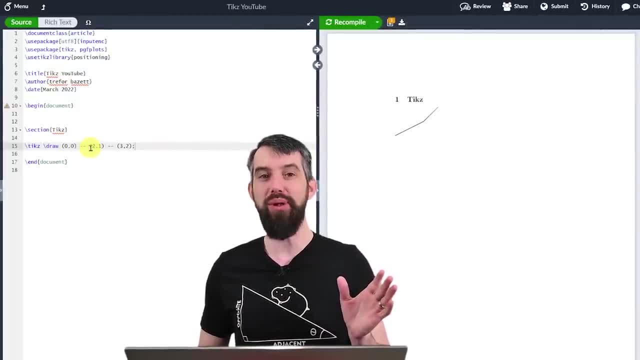 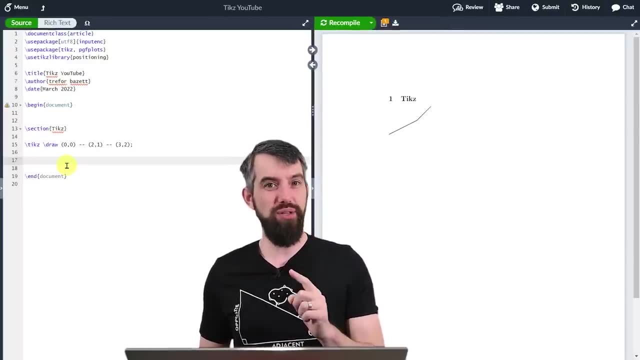 I could add as many of these as I so wished, with this little double dashes to indicate that I wanted to create an idea and find some lines. Now I want to jump to circles, But they're actually multiple types of circles, So instead I'm going to do myícula first, then fore under either of them. 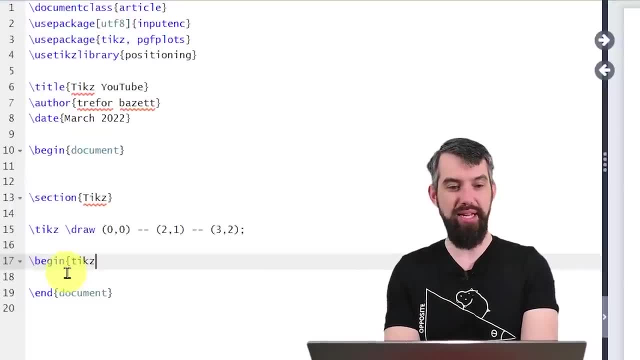 So instead what I'm going to do is I'm going to go backslash, begin and I'm going to write tixi picture And notice that what happens here with overleaf is that it pops this button. it recognizes what I'm saying. So if I just hit enter, It'll actually come and nicely format the beginning and the end point here. It'll actually come and nicely form the beginning and the end point here, the end point and then down the end point- fluorescence function. So if I just hit enter, it'll actually come and nicely format the begin and the end point. that. 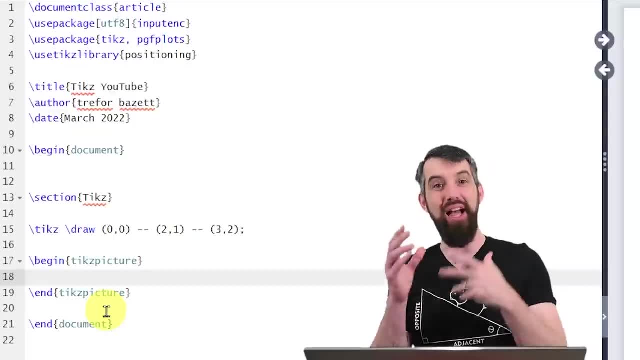 end text picture. It just saves me a little bit of typing. It's kind of like a little predictive pop-up. Okay. so I want to do the same kind of thing here. I'm going to draw, And the way it works is: initially I put in the coordinates of the origin here, So I've gone and put in 00 to. 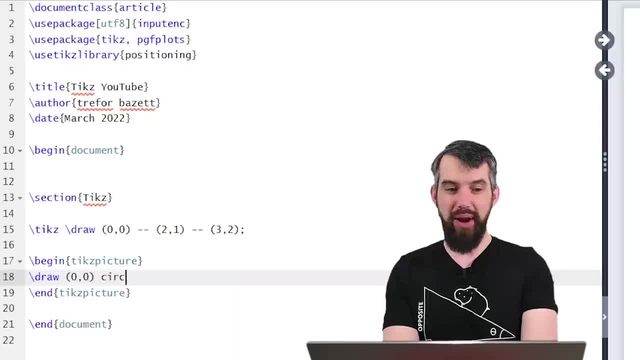 say that it's going to start at 00. And then I write that it's a circle. This is in contrast to previously. I'd written this double dash here. Now I'm going to write circle to indicate that it's a circle, And then I need to put in the radius of the circle. And I have a few options. 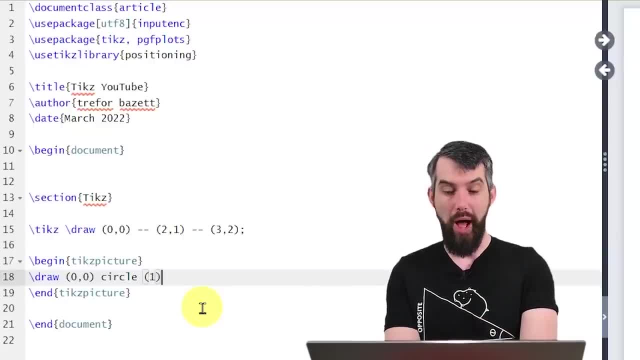 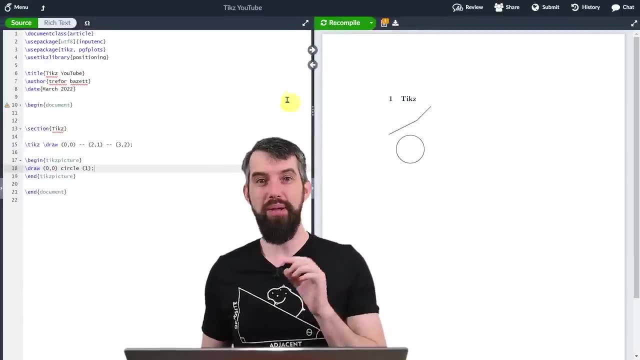 for doing this. If I just write in, for example, 1, let's just see what happens. if I do this, This is going to make a circle of radius 1.. But what does 1 mean? Basically, there is a default. 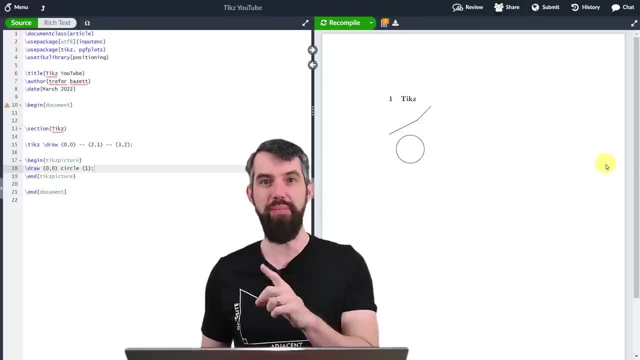 distance scale. that's going to here. We'll see how to change it in the beginning, But right now we'll have a radius of 1, corresponding to, I believe, to 1 centimeter here, And nevertheless we get this nice little circle In contrast, let's do. 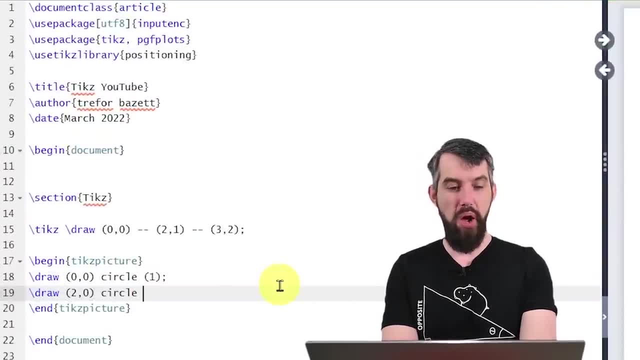 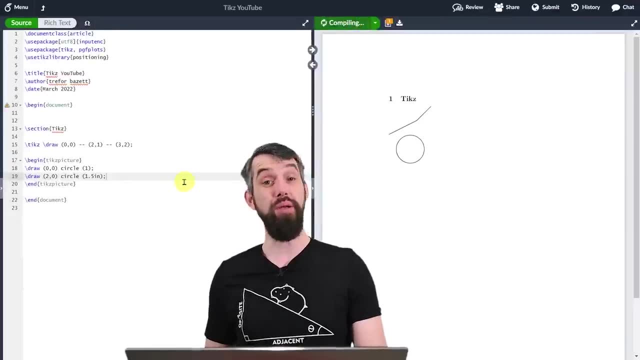 oh, I don't know, maybe I'll start it at 20.. So it starts at the right. In contrast, let's do this radius as maybe 1.5. But let's write it in terms of inches And we can recompile and see what that. 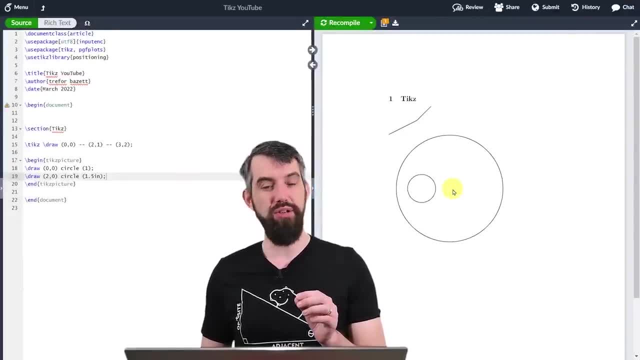 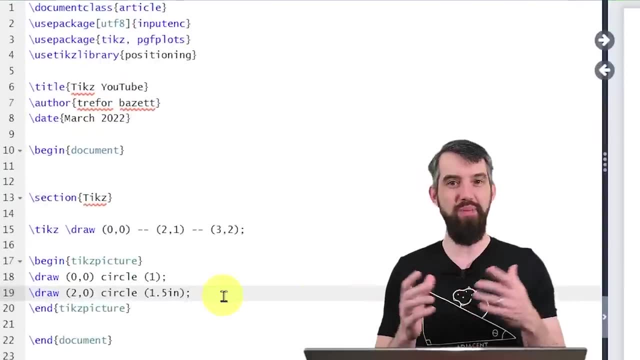 does. This now is a very big circle, So it starts at 20.. So off to the right here, And 1.5 inches for the radius is a relatively large number. It makes this big circle, So you might like to use. 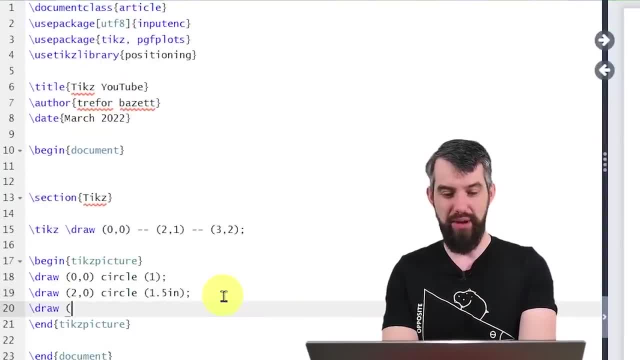 one or the other I could also draw. let's do it over. how about like at 50.? This time I'm going to do an 11. Ellipse. Oh, I have to spell ellipse correctly. It lets me know. I forgot the extra L And an ellipse. 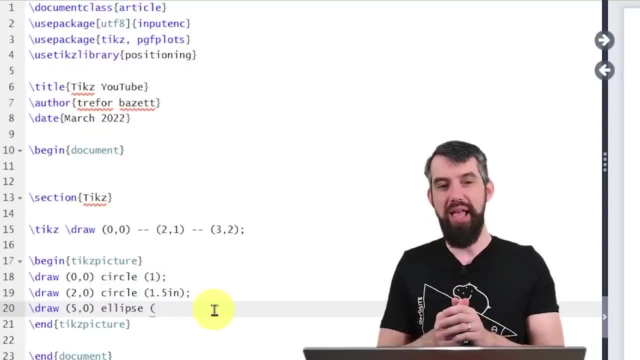 has two different radii, a major and a minor, And this one- maybe I had previously done it in terms of just no numbers and then inches, But this one, how about I do 10 point and 20 point, something like this, where this is the same sort of size that you imagine when you're thinking about like 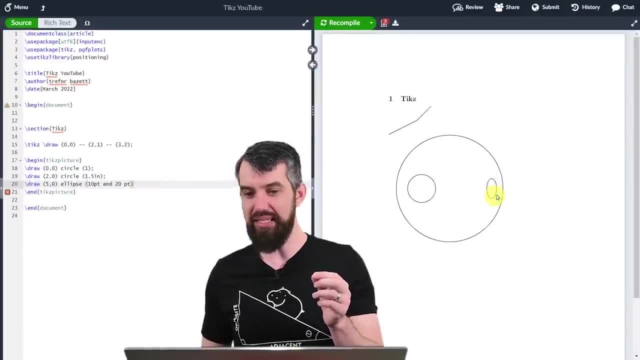 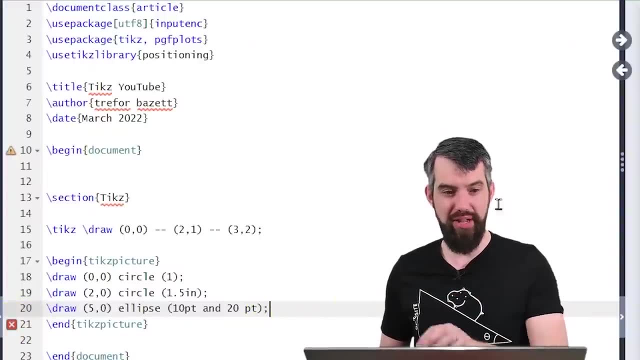 a font size And so nevertheless it gives me this nice little ellipse over here. Notice it says that I can hover over it. It says: did you forget a semicolon? Yes, I did forget a semicolon. So Overleaf is really nice at being able to manage your errors and figure out what it is that you've. 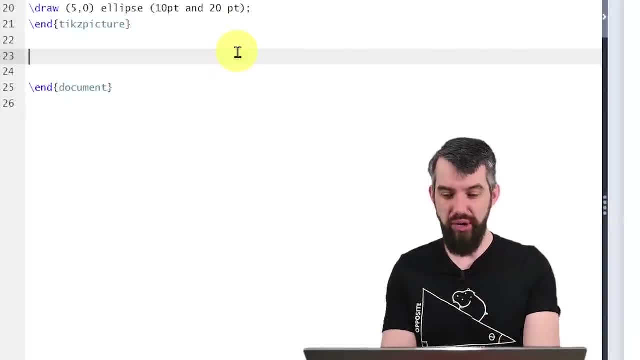 done wrong, So that's line circle ellipses. How about we do a new one? I'm going to do a new begin Tixie picture and just quick hit the enter to auto-complete that I am going to draw now a. 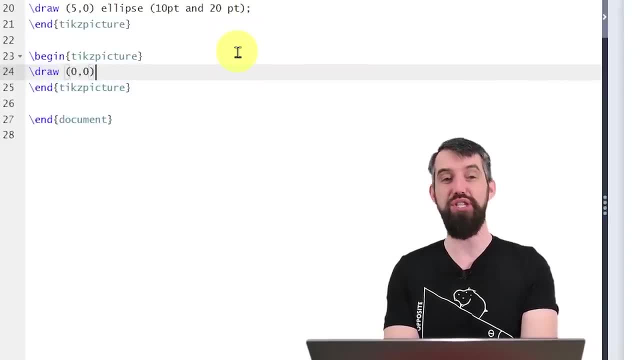 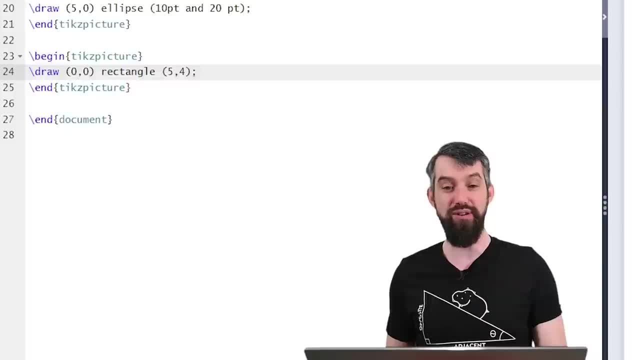 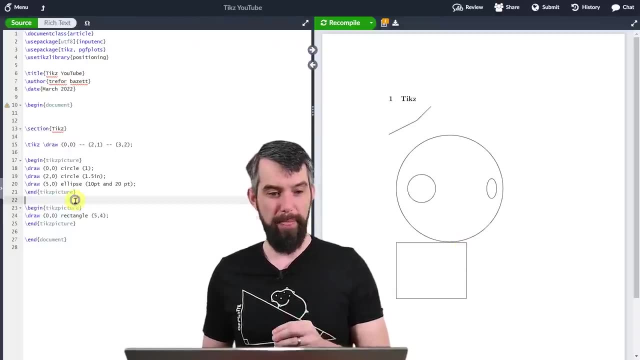 corner 54. These are like the two different opposing corners of it, Something of this nature, And it's going to make me a very nice rectangle going from 00 up to 54. If I didn't want it squishing, I could come in between these two things and make, say, something like V space one. 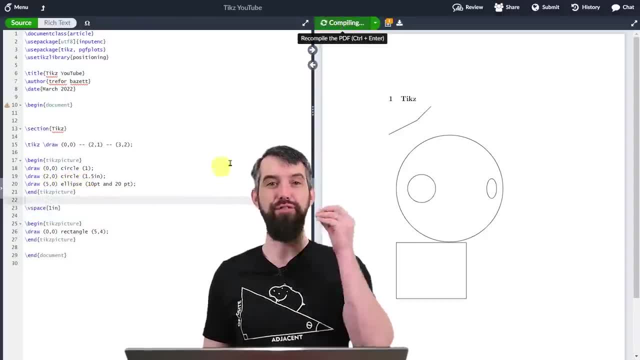 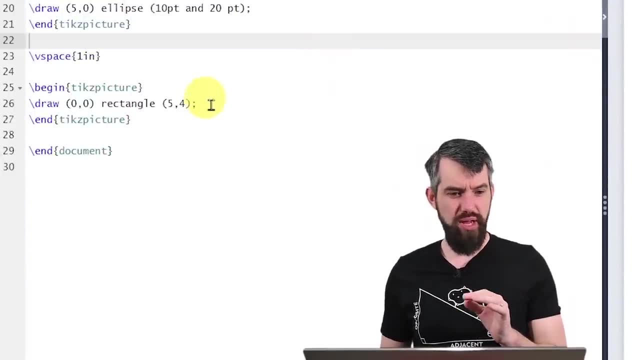 inch, And that would give me a sort of a forced input of one inch of space between these and get this nice little separation. Final primitive that I'll show you here is: okay, I've got a rectangle that goes from 00 to 54.. But you can also do something called a grid, And in this case 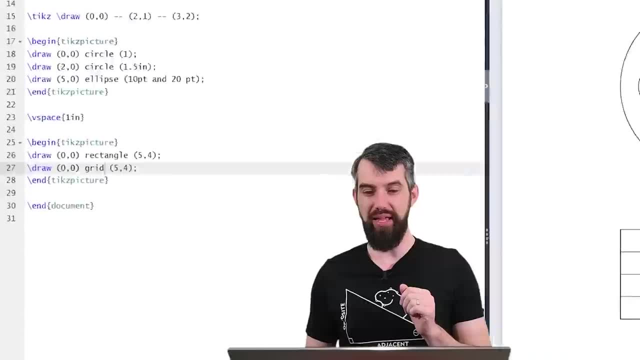 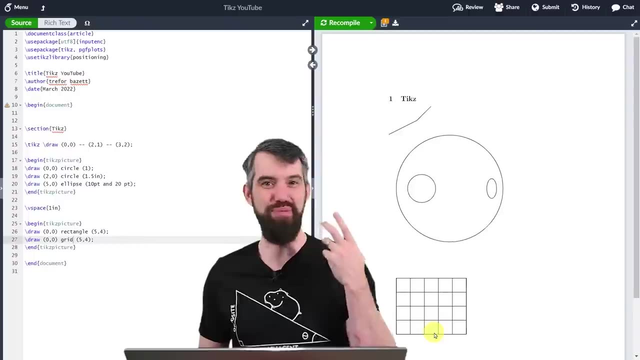 the grid is going to fill in that rectangle. Let's see what happens when I compile it. It fills it in with a spacing of one And I'll be able to adjust that spacing. I'll show you how to do all these kind of adjustments of color and style and spacing and all these different things. 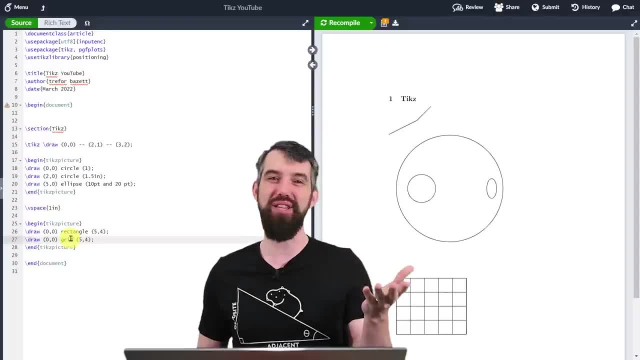 in a moment. But the point is, a grid fills it in, And this is just really useful, As you can imagine, if you're trying to, you know, draw a graph of something. you want some, some nice grid on the background. Okay, 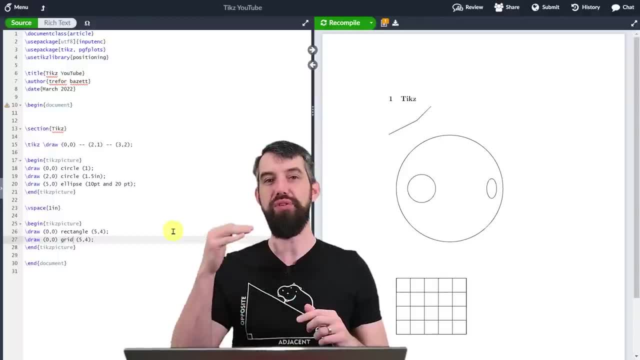 So what I've shown you thus far is a lot of the sort of basic primitive objects that we can created, like lines and circles and grades and rectangles, But normally you don't want them to all look the same and all look black and white. You might want to have color and style and all. 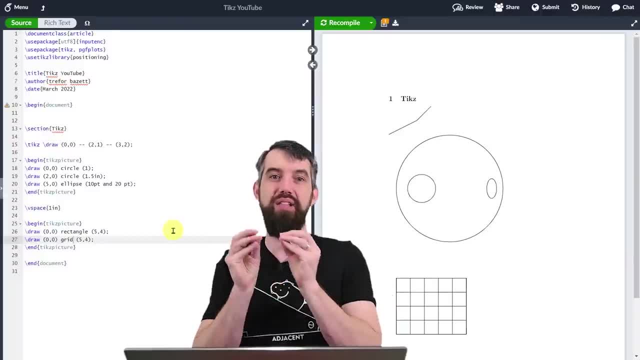 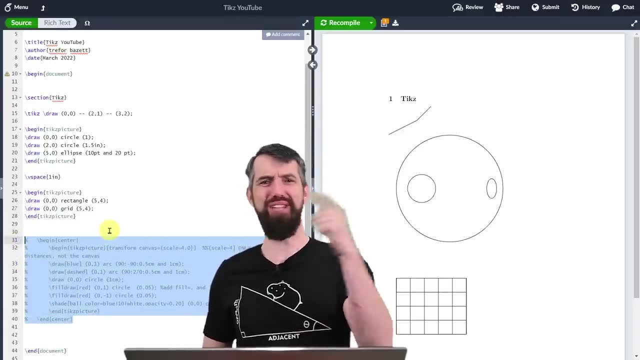 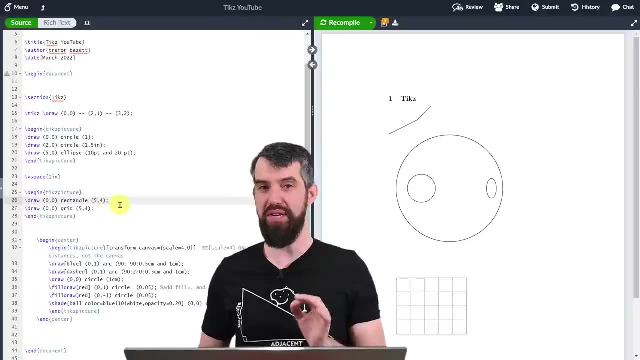 sorts of other things. So I want to show you how you can modify these basic primitives. So how I do this. I've copy and pasted some code that I actually had to use in a presentation. I've done. I'm going to select it all and do control slash to remove the commenting from it. So this is the. 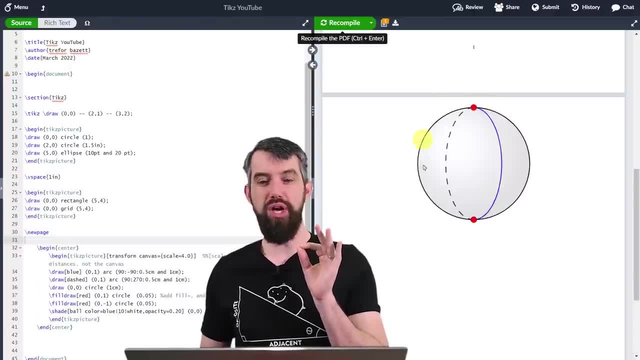 image that we have a little fancy, what we've seen before And I want to walk through the code to be able to make it Now. the first thing you'll notice is that the begin Tixie picture and the end Tixie picture are wrapped in: begin center and end center, And I often do this with my graphics to have them. 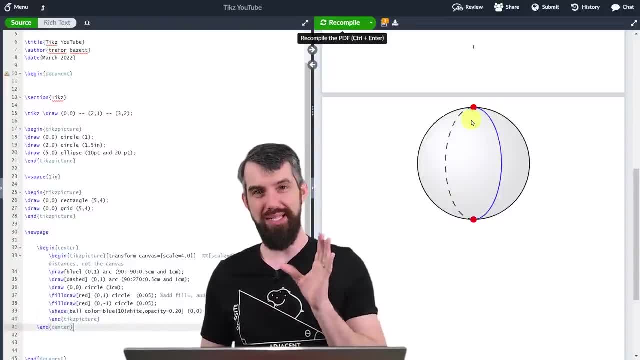 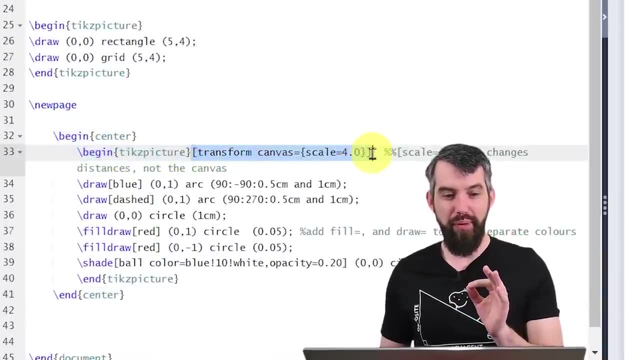 centered. We've seen this kind of idea previously in the series, So I've put this in the center. The second thing I've done here is in the middle of the picture I've added a little bit of a scale. So when I do begin Tixie picture, I've added a parameter where I transformed the canvas. 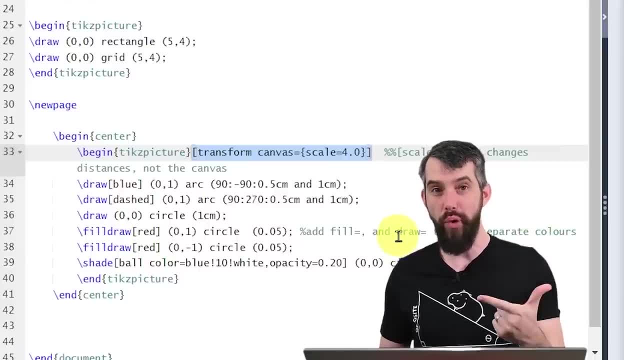 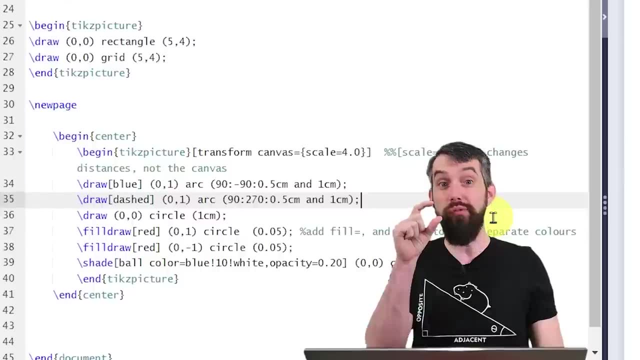 and scaled it by a multiplication factor of four. So basically, we had previously seen a scaling where, you know, the value of one was a certain distance. in this document, Now that I've scaled it, that value of one is going to be four times larger, And that's useful to be able to make these 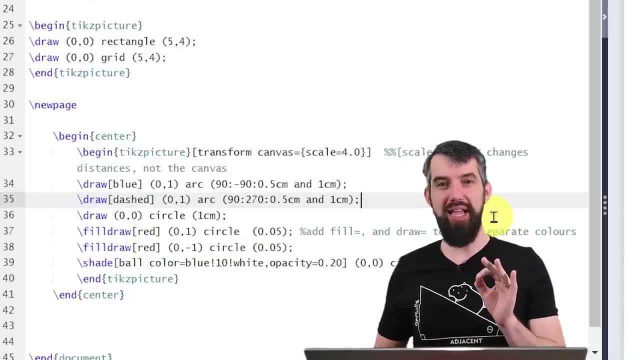 nice large things. When you do transform canvas, everything increases. So, like the thickness, for example, of a line is going to increase. If I didn't do this, let me just take off the transform canvas. This is very common, you'll see. this is just a scale equal to four. it is almost. 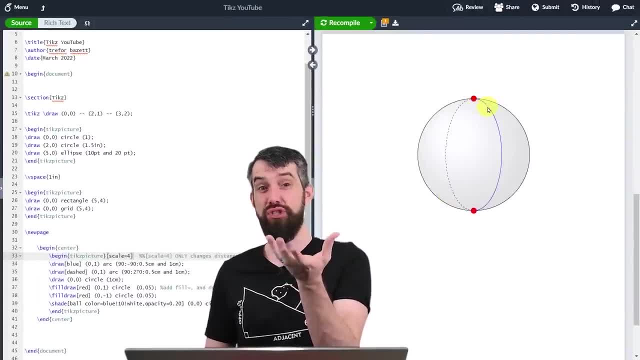 the same as in. it's four times larger the the inherent stretching of the base canvas has still gone larger, But everything just looks a little bit thinner than it did before. And this is because when you do scale opposed to the transform scale, it's not just blowing up the entire image. 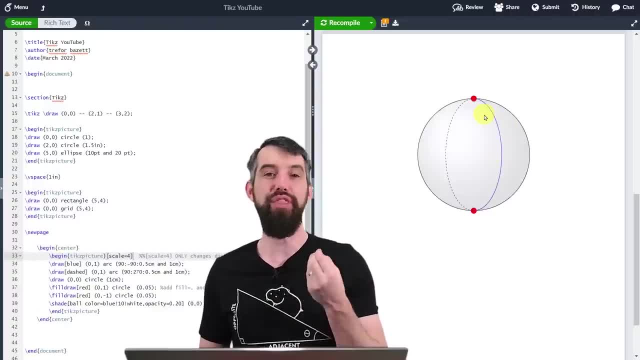 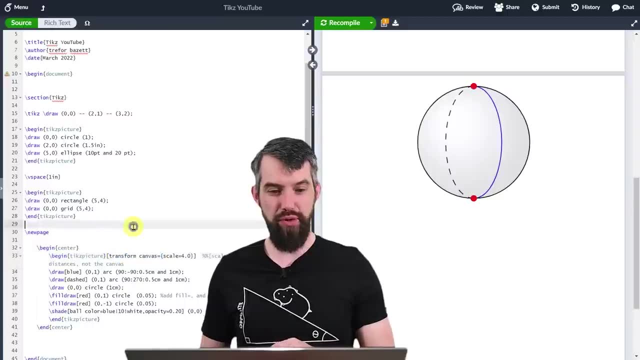 including the thickness of everything. It's drawing things that the default thicknesses would have before, So I'm gonna go back to transform canvas so that things look a little bit thicker, Okay, so now let's go through what's happening. First of all, I noticed that this arc 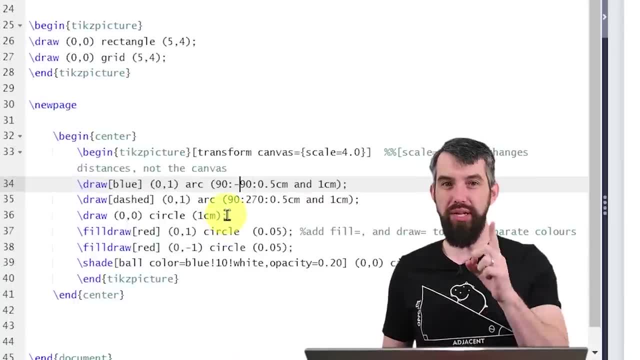 here is not black, it is blue, And basically the way this works is you put in square brackets properties of the object that you want to impose. So, for example, draw blue, that's creating this blue arc. draw dashed- that's creating this dashed arc. If I wanted to do, for example, dashed and 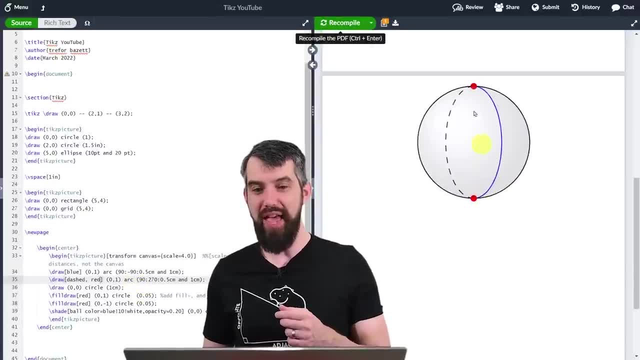 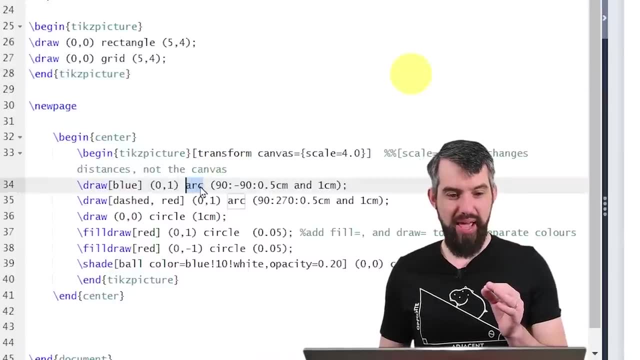 red. I could just put that in, you know a comma between them, And then it will go from dashed and black to dashed and red. You'll also notice that I'm drawing arcs, And the way I do that, by the way, is the same sort of idea. I put the center point. 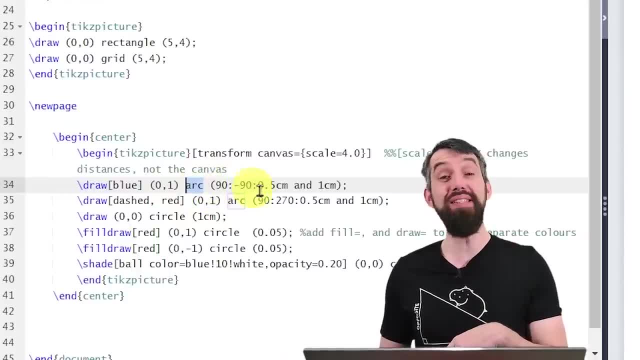 in. then I write arc as opposed to circle. This tells me the degrees going from from 90 to minus 90. And then, because it's actually part of an ellipse, I have to give you the major and the minor which I put: a half centimeter, one centimeter. The next thing is how I've got this. 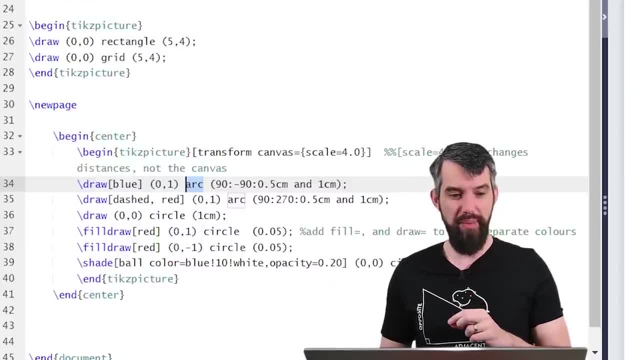 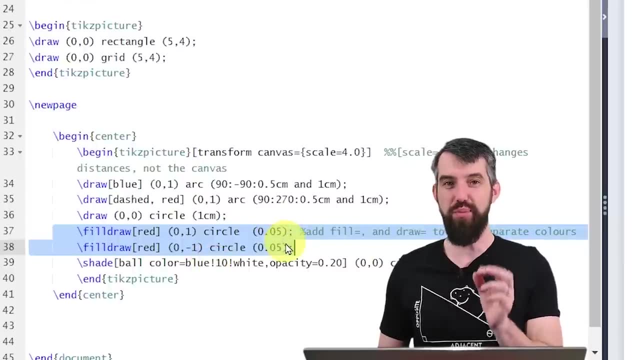 red filled in circle at the top and this red filled in circle at the bottom. So you'll notice, both involve circle, exactly we saw them before- circles with a very small radius, But what's different is that they're filled in. So what I've done here is, instead of doing backslash draw, I've 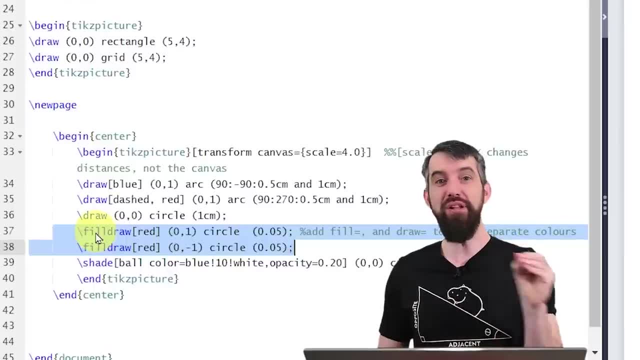 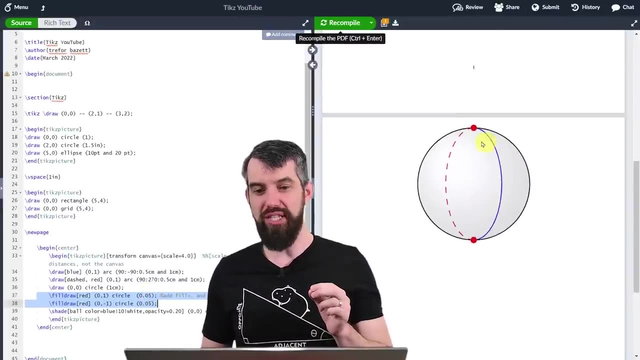 done backslash, fill draw. and fill draw says it's going to draw the outside and fill it in. If you just do draw it just as the outside, if you just do fill it just as the inside, fill draw does both of those. So I fill those in with red And then the final thing here is: you'll notice this background. 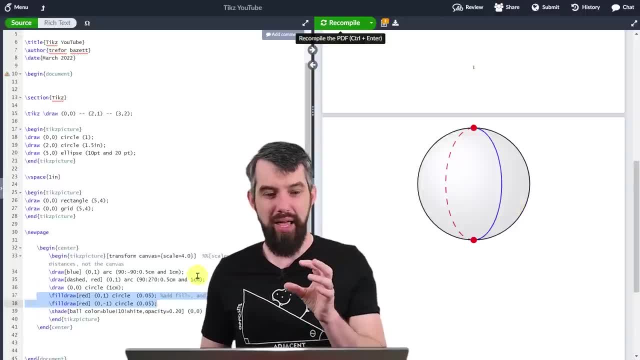 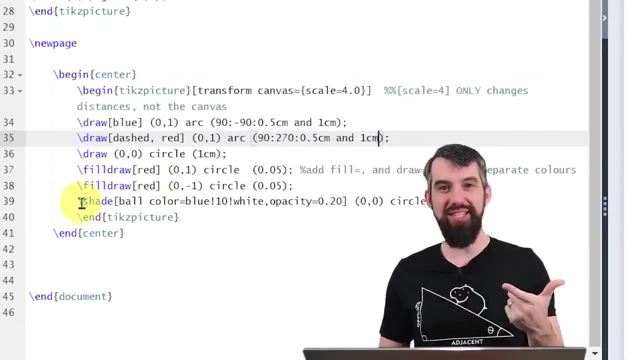 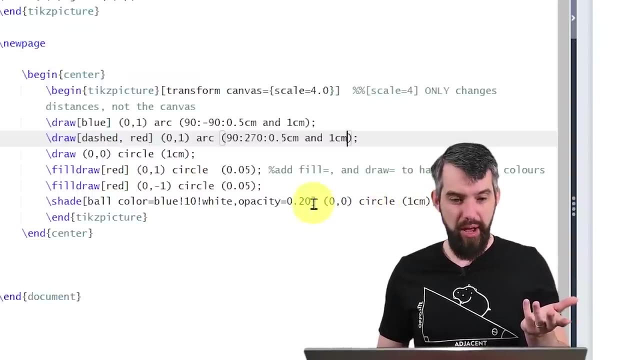 ball is just great, sort of like a nice shaded gray, And for that I do backslash shade as opposed to backslash fill shade is going to have this sort of this nice little gradient that is going to be imposed on it. Other than that, it's just a circle with a center and a radius, But I have a bunch of 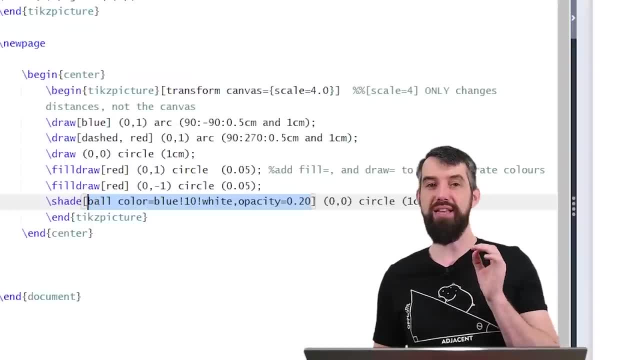 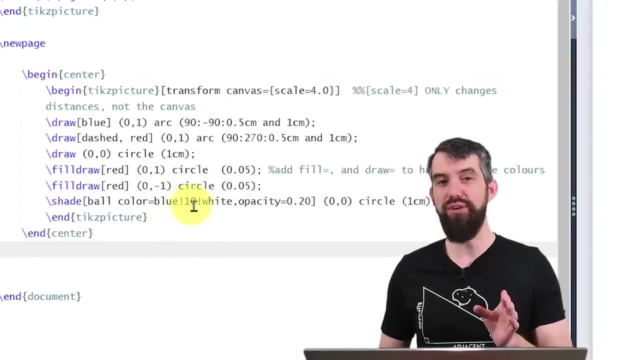 different properties that I've put in here for that, for that shaded object. So in this case we've seen this notation before, where you put two colors and then you put the percentage. So this is going to be the percentage of the color, And then you put the percentage of the color, And then you 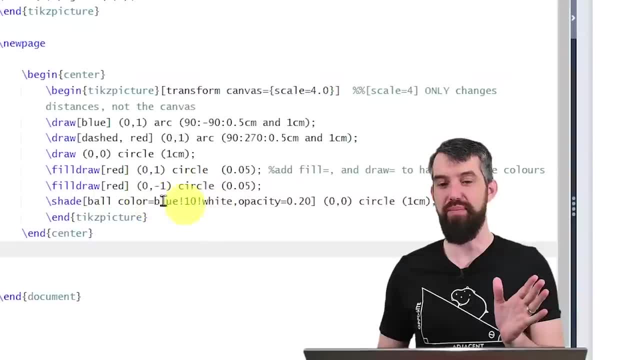 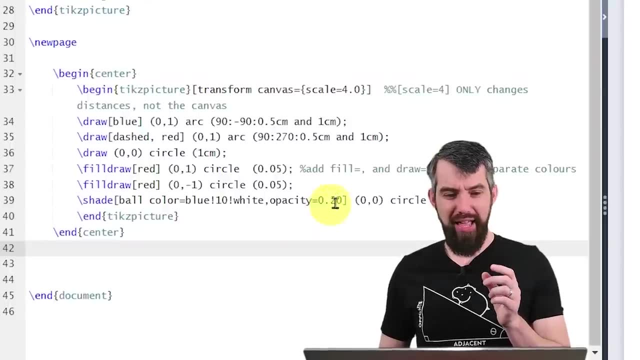 put the percentage of the color, So this is going to be 90% white and 10% blue is sort of this mixture between it. So it ends up looking relatively gray in the end, but but actually got a slight bluish tint to it And then, if I had not added this opacity, this is actually a little bit of a hack. 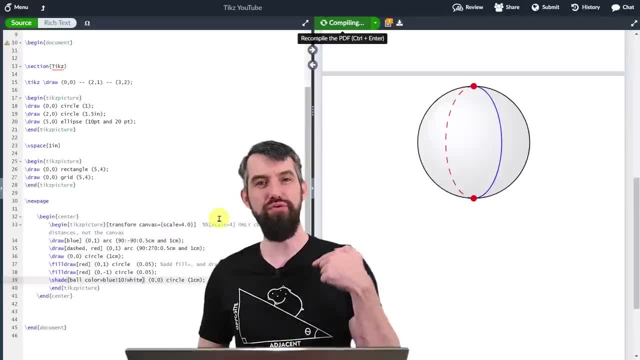 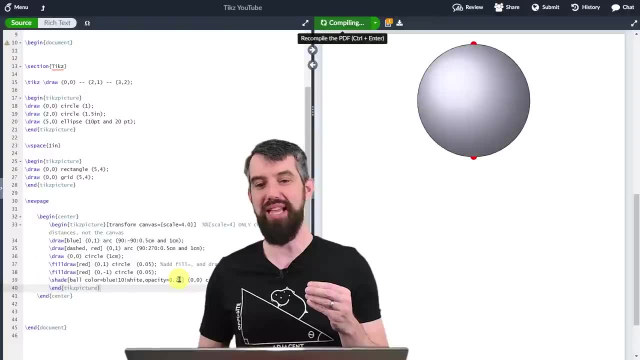 that I did it this way. If I did not have the opacity there, it would have drawn on top of everything else. So you see how it would draw on top of it, And so I also added this opacity of basically 20%. But put it over top of everything could have been cleaner. just to list it first. 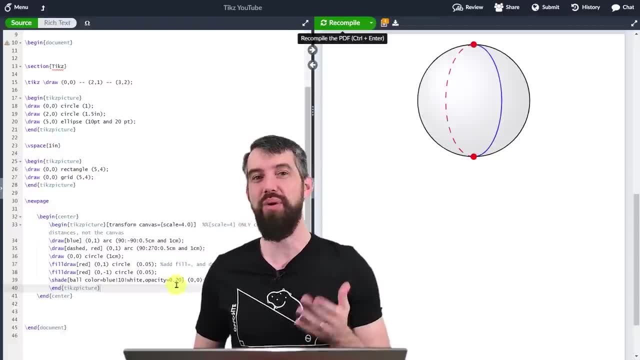 without adding this opacity. And then if I had not added this opacity, this is actually a little bit of a little bit of an opacity, and then everything could go on top of that. But either way is going to work out fine. I actually want to do a couple more properties. I'm going to go back to the very 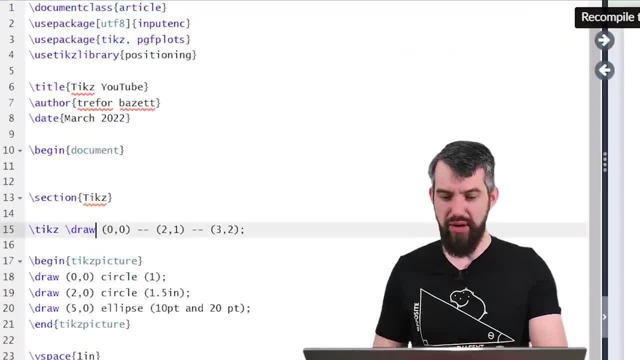 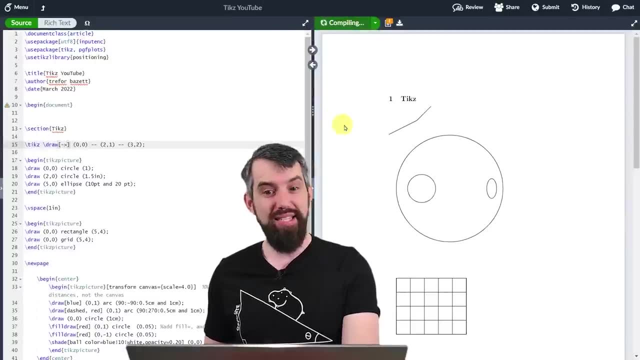 beginning here. Notice how I have this draw. I want to show you how you can make it into an arrow. you literally just put in your square brackets a little miniature arrow. If I do this, then I'm going to have it appearing to be an arrow at the end. I could adjust things like the size of the. 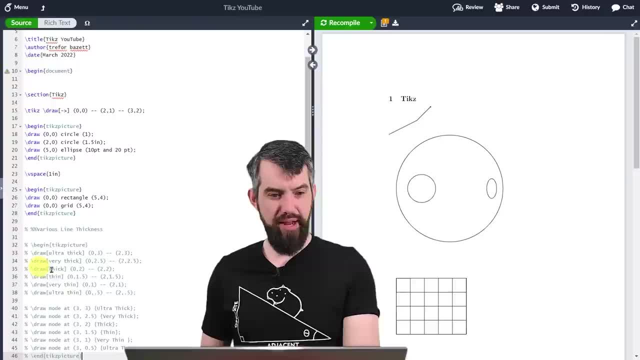 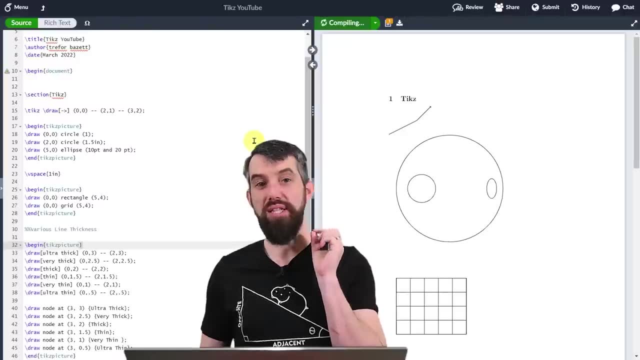 arrows if I so wished. Another thing I can do here is I'm going to copy paste another block of code that I've previously written on. This shows me how I can do a bunch of different line thicknesses, So it looks very complicated, But 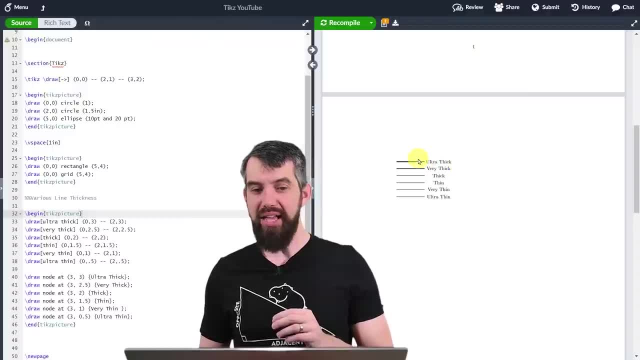 all I'm doing here is showing that I can. I can go into my draws. I've just done a bunch of different lines And I can specify one of ultra thick, very thick, thick, thin, very thin and ultra thin. So I 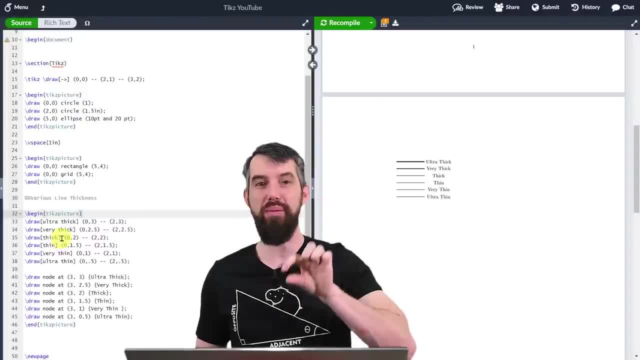 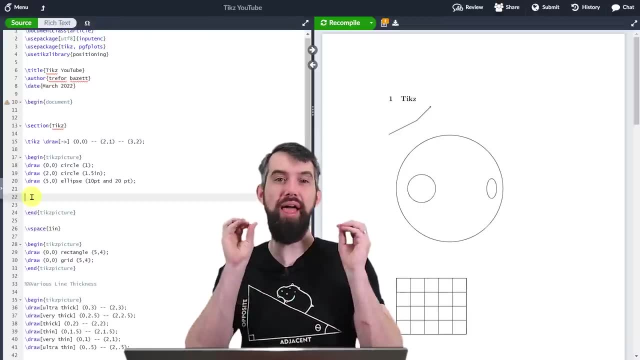 often like to adjust the thicknesses of my objects in this way. So I've showed you a lot of these primitive objects, But I want to show you an incredibly powerful one, now called a node, And you can think of a node as like a spot in the document where stuff can happen and that you 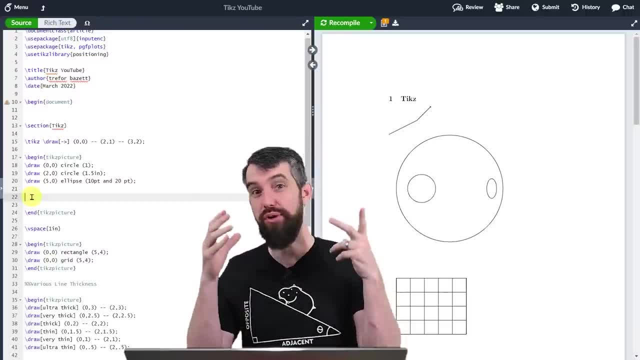 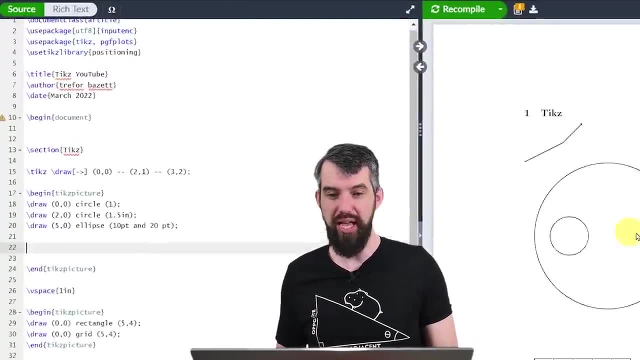 can relate back to it. Maybe you want to put text there or you want to put some sort of object. So I'll begin with the simplest, which is just putting text at a specific place. Like let's go back to our one with our three circles. Maybe we've said okay at 00,, 20 and 50, I have something Okay. 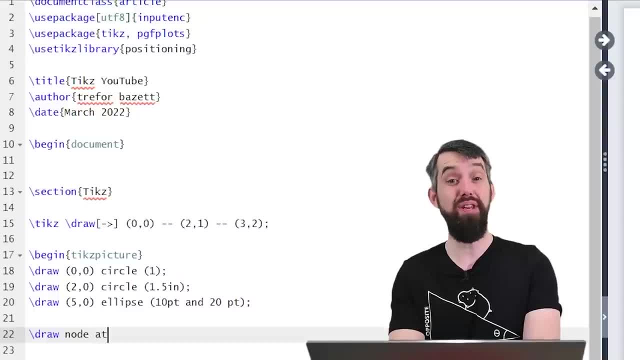 so my syntax is: I'm going to draw it again, I'm going to write a node and I write, the node occurs at a spot like, well, I don't know how, about three zero? And then I'm going to put inside the 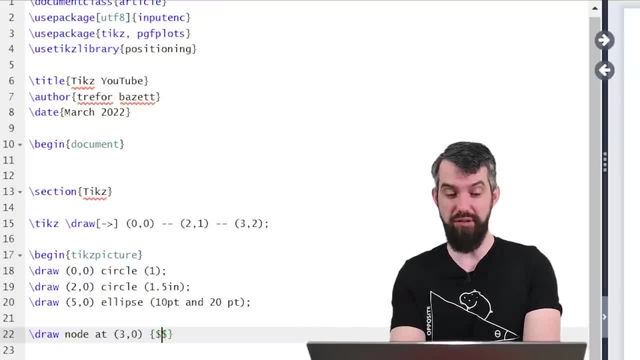 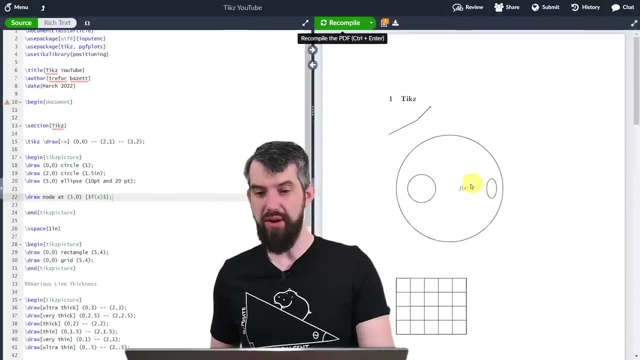 squiggly brackets. whatever, the text that I want to display is: how about I do some mathematical text? I'll write f of x that's going to occur at this particular spot. I'm going to recompile and let's see what we get. So right here, at that value of three zero, we get this f of x And actually 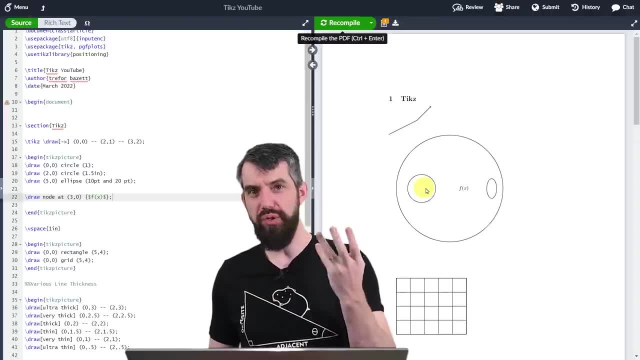 this spot where you might start really preferring to use Tixi over just like any other image editor and then add your graphic in as an image, Because if you were trying to do this- and I don't know- a lot of the maps I just draw are a big. 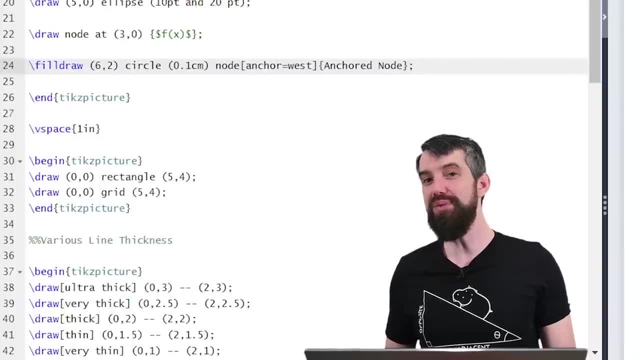 that shows this is going to be done in a little bit of a different way. So what I've done here is I've done a full draw that fills in that circle and I'm going to make a nice little filled in circle at the value of 6, 2 and uh, with a radius of 0.1, doesn't matter. now, this is the interesting part. what I'm going 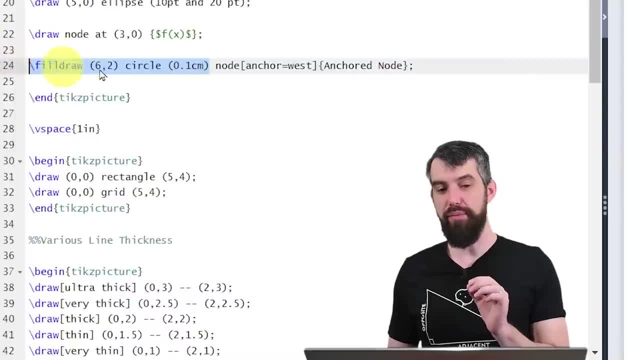 to then do so. so so this part here is all something I might have seen before, but then I'm going to append to it a node and notice what I've done here. I say node and its anchor is to the west of it. so basically, what we're imagining is that this circle is to the west of the node and then inside. 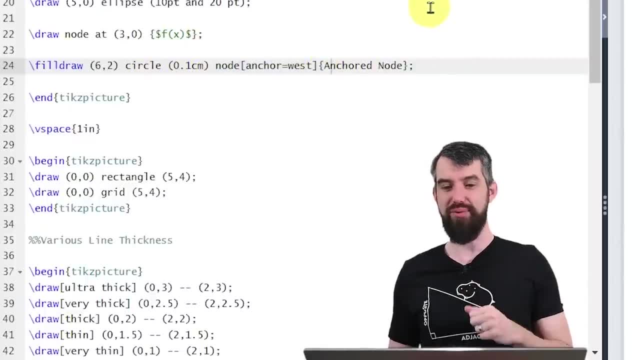 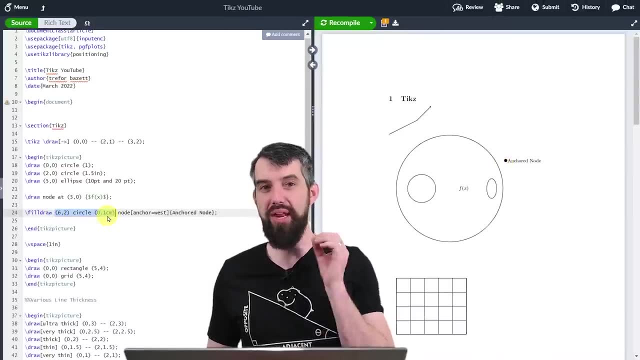 of the node. in the squiggly brackets I write anchored node, because that's just what I'm trying to do. I'm trying to demonstrate an anchored node. so what do we have over here? we have that little bullet point appearing. that's what's created by this nice little circle with a radius of 0.1. 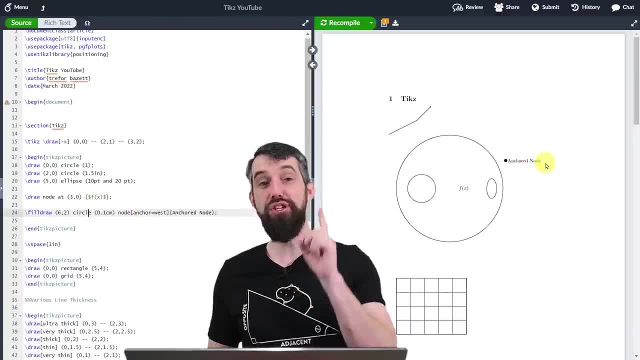 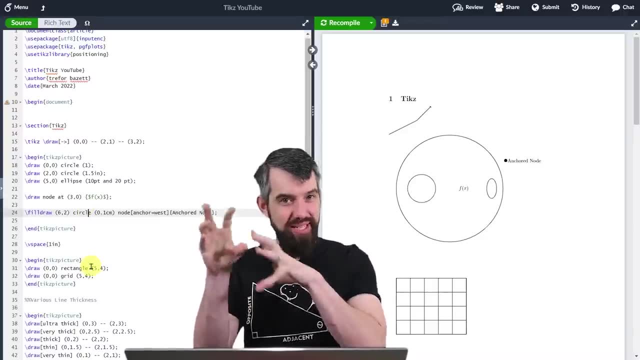 centimeters and and this node has to its west the previous circle that was mentioned. so this is kind of a way that you can attach one item, this, this text, to something other thing that you've talked about and I don't have to then change it. I don't have to always move. 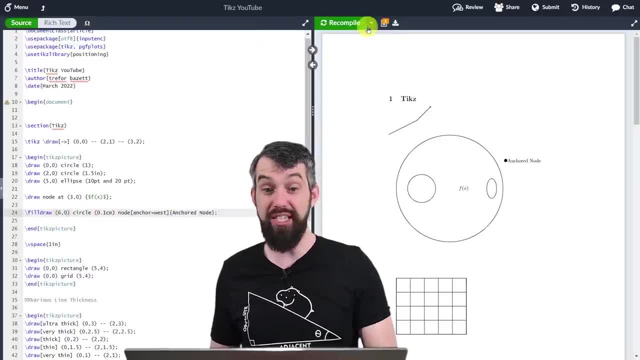 the text around. so, for example, if I go from 6 0 or 6 2 rather to 6 0, so it's going to move it down, I don't have to redo the text. that text because it's a node that is anchored to this particular. 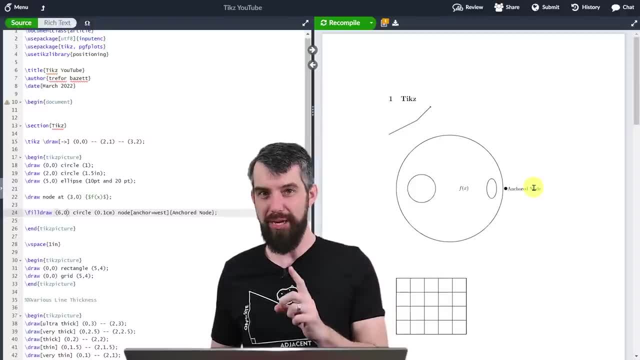 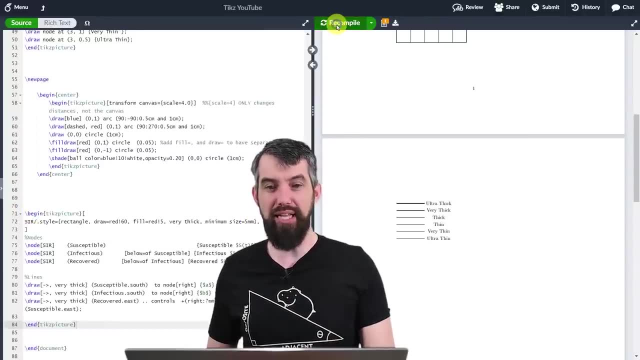 circle. it just moves along with it. so very powerful way of doing it. but notes are actually more powerful than even that. I'm going to go to the bottom and I'm going to copy paste some code that I've done before. let's first just compile it and see what we're going to get. okay, so this is. 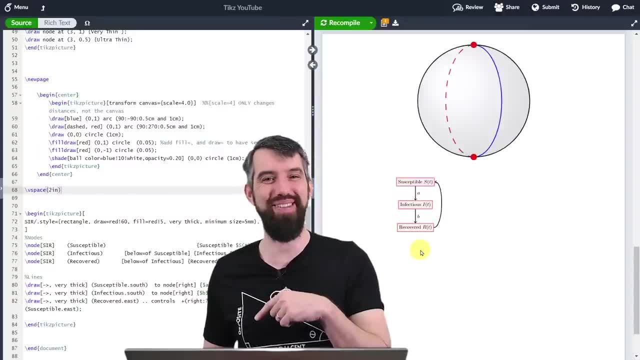 the nice little diagram that I have. if you've seen my previous videos on the, the sur model for pandemics, you will certainly recognize this diagram. but this is the diagram I want to take and what I notice about this is I have some various text and some, you know, mathematical. 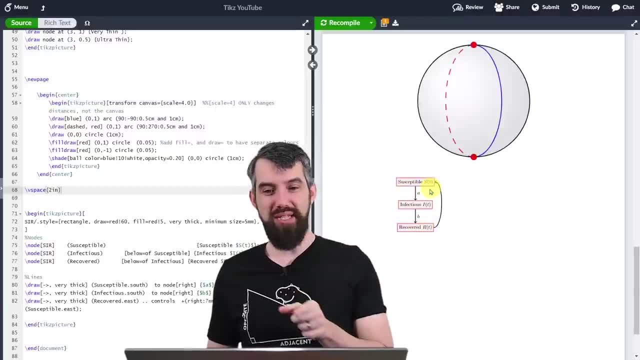 symbols here, but I wanted to surround those text in these nice colored boxes, have arrows going between them. that's what my objective is, and and doing it with nodes is way easier than doing it with kind of the the static rectangles and arrows we've seen above. let me show you what I mean, okay, so? so this is the code that I've added. 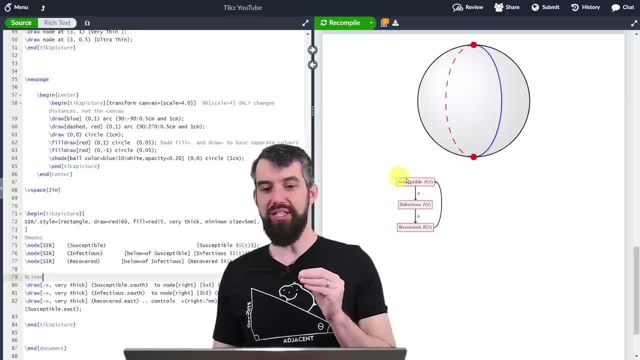 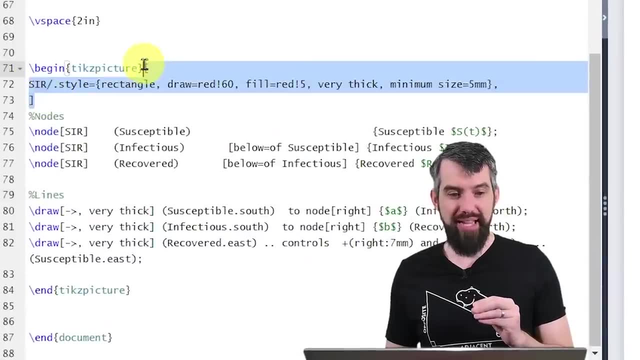 to create the subject, the. the first thing I notice is that this red box repeats itself three different times, and so I begin, in the tixie picture, by specifying the style of something. so I'm going to create something referred to as sir. this is called the sir model of the. 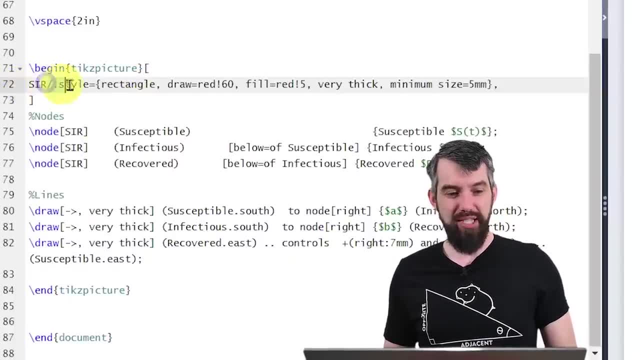 uh, for pandemics, and what I'm going to do is I'm going to specify its style and I'm going to put in here all the brackets about this. okay, so what is it? it's a rectangle. so so the idea is you have your node and then whatever you put in your node, it's surrounded by a rectangle. this is what I mean. 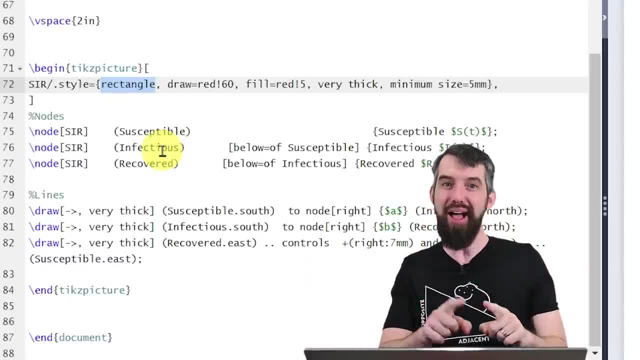 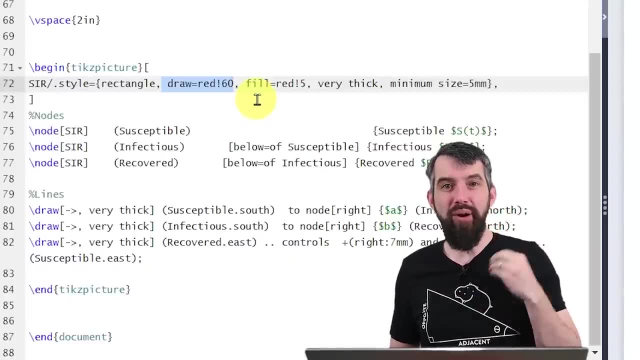 by a style of it. it's different than drawing a rectangle. I'm saying the style of this node is a rectangle, the draw portion is the boundary and I've set it to be very red. I specified it here to be 60 percent red and and 40 percent red and I'm going to put in here all the brackets about this. 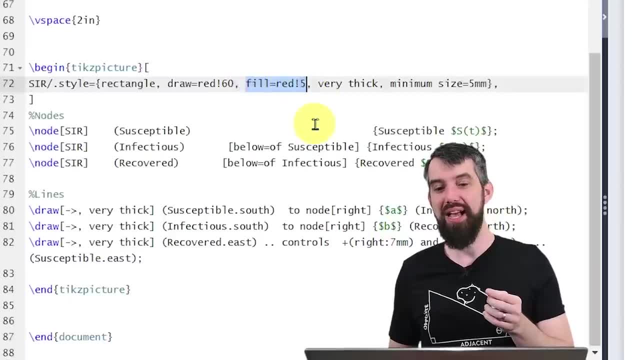 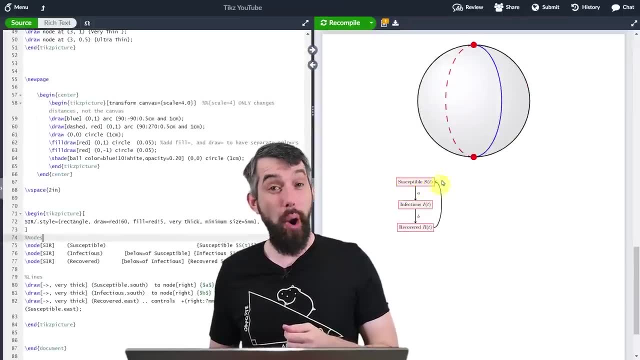 and I'm going to put in here all the brackets about this. in contrast, the fill which goes inside, I've set it only to be five percent red and and, uh, 95 percent white. so this is why you get this sort of really nice dark boundary for the, for the draw, and then this light for the fill I've specified. 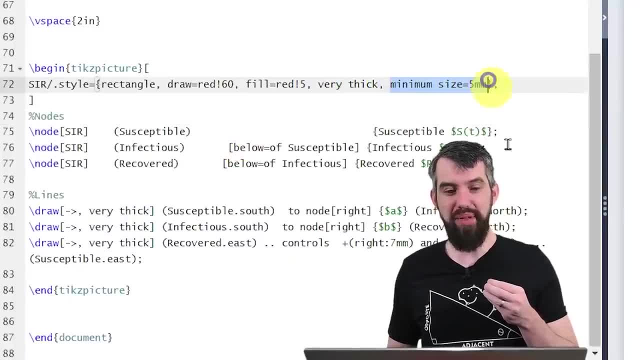 its thickness to be very thick. and then I've also done something kind of special here. I've said minimum size of five millimeters. the idea here would be, if I put nothing in for, say, susceptible here, the smallest box that would be drawn would be in the middle, and then I would put in here the 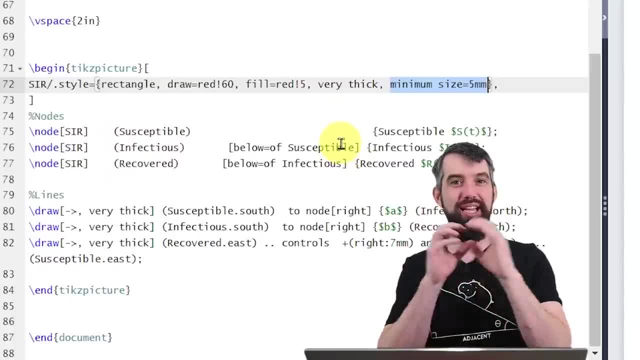 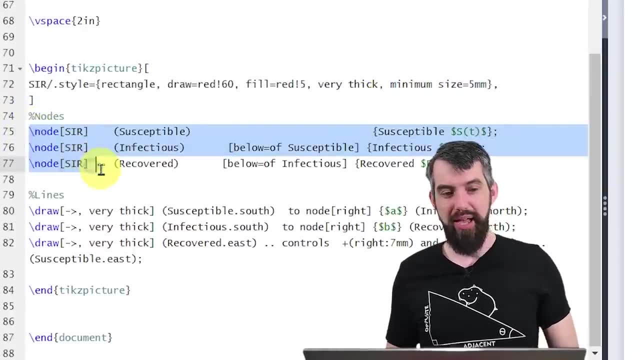 nice little rectangle, you know, with five millimeters along the outside edge. it's basically saying you have to have a minimum size to the node anyways. so those are my styles. okay, now let's what I've done. I have created three nodes. each of those nodes has as a parameter SIR. so I'm saying I'm 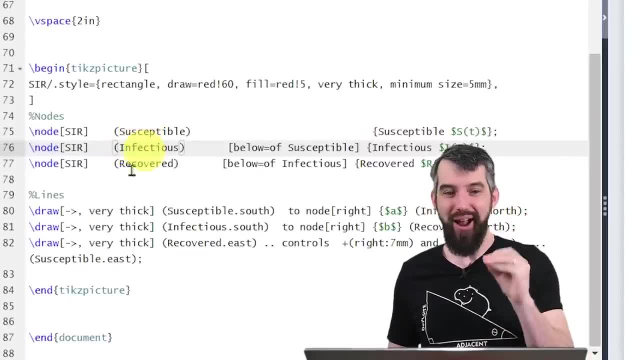 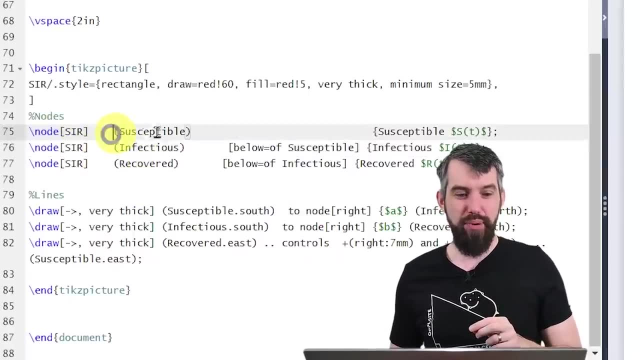 drawing a node of the style, the SRI style, which is this thing with this fill and this draw and all that, then it's quite interesting. here. the next thing I do is I put it in round brackets: susceptible, infectious and recovered. these are not the same thing as the SRI style, which is the SRI style. 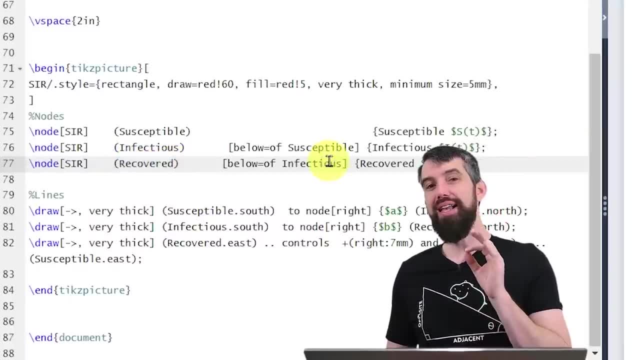 not the word susceptible, infectious and recovered. this is the name of the node, so it allows me to refer to that particular name coming up in the future. okay, so then, so this. so the way I read this first line is: I'm creating a node of the type SIR that is labeled susceptible and then over here. 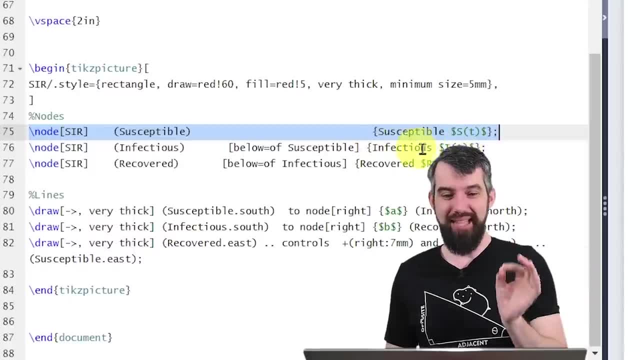 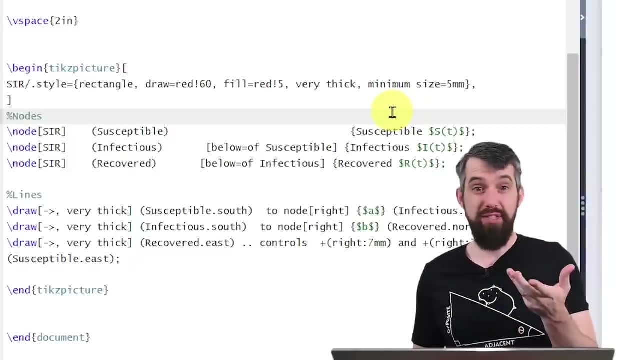 in squiggly brackets I put what's actually displayed susceptible, and then it would number signs S, of T, so that's what's displayed here. now I haven't put any localization in here, so I'm just going to put it in the first location. I've just said: spit it out at the default first location. 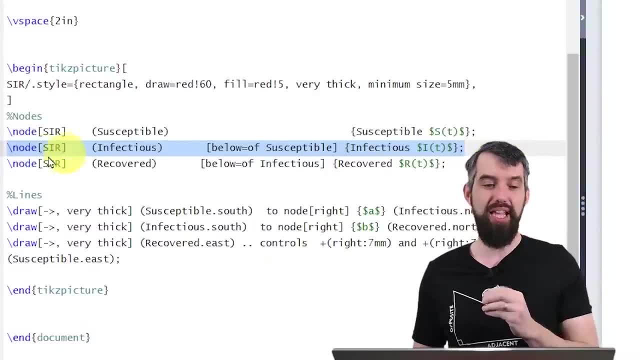 but notice what happens for the second thing. it's almost exactly the same. another node of type SIR. it's called infectious this time and in the squiggly brackets it's got the new text display: infectious, I of T. but I have here this section in square brackets and I just say below is equal to: 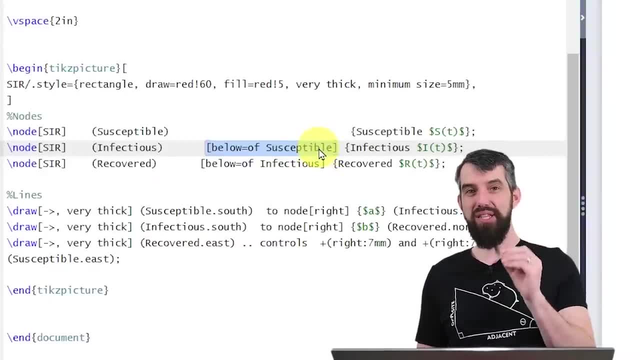 of susceptible, and what this does is because it's a node, and nodes are all about relative placements here. it allows me to take the susceptible and the susceptible and I just say: below is equal to of susceptible and below it is where it's going to draw the infectious. you could have also written: 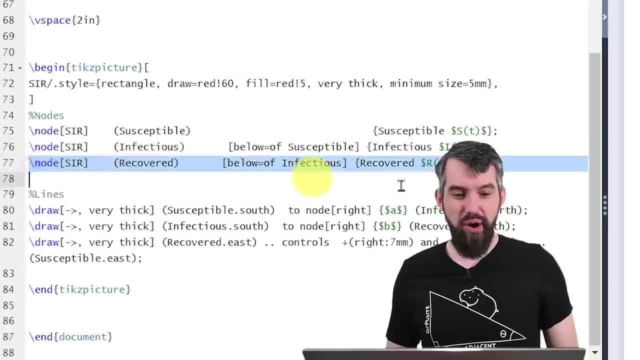 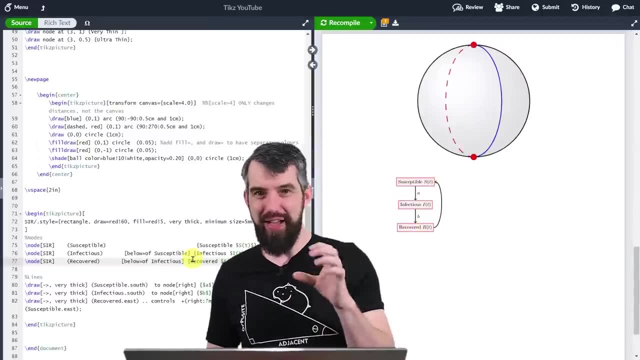 to the right of it or anything else like this. okay, then I'm going to add the third node, which is the recovered node. it's going to be below the infectious and I spit it out here, if you want to. you can specify some of these distances between them, but- but, this is just sort of the default and 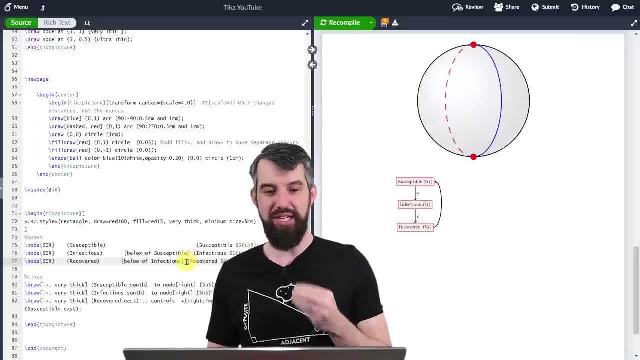 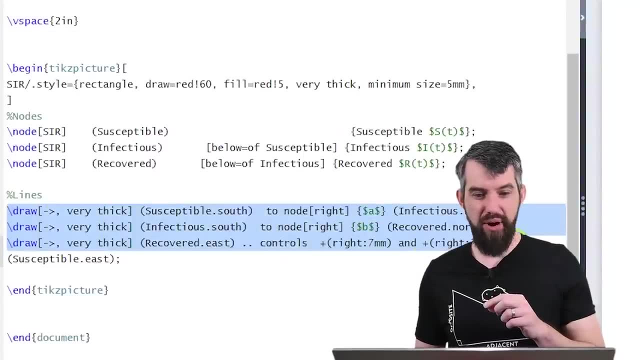 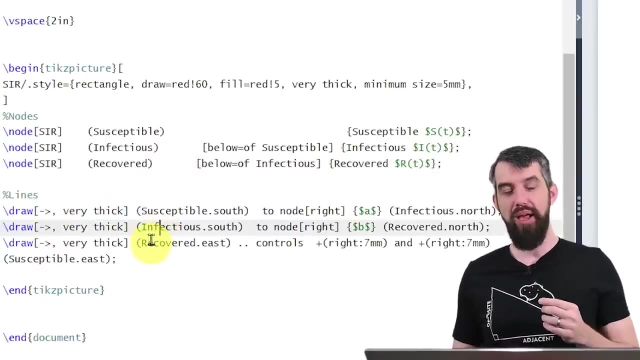 what's nice is, if I move things around, the relative position is going to be the same. next up in my diagram I have these little arrows. I have to deal with them, so I've just done three arrows. they're just the same. so I'm obviously going to be using the normal drawing of a, of a, of an arrow that happens to be very thick, that we've seen before, but instead of putting the two locations as like 1, 1 and 2, 2 say the things I put in the round brackets for their locations, which is here, and here is in reference to my previous nodes. so this a arrow which is to go from the south side of susceptible to the north side of infectious. this is how I do it. the first one is susceptible dot south. the north one is the infectious dot north. 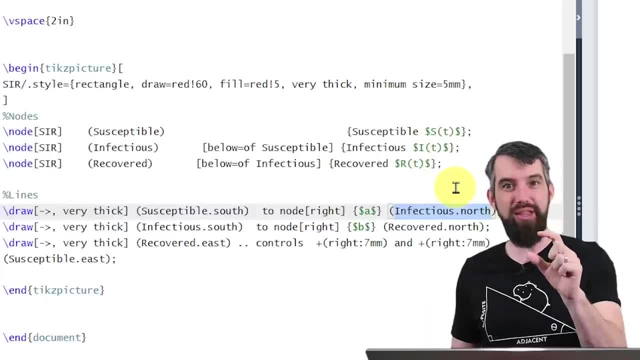 the other one is theców sepSEPTIBLE dot south. the north one is the infectious dot north. So I'm not putting like actual specified locations, I'm making everything relative, which allows me to adapt and tweak this diagram as many times as I want to. 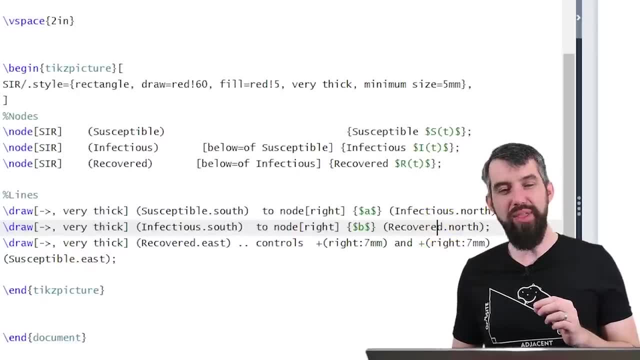 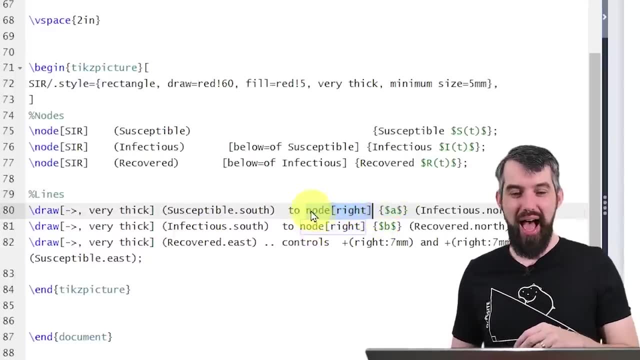 The final thing is it's not just an arrow, It's an arrow with an A beside it. The way I do this is just I stick in a node here that in between the one location and the other, I say that I want to make a node. It's to the right of the object that I'm talking about and it's going to be this: this number of A. 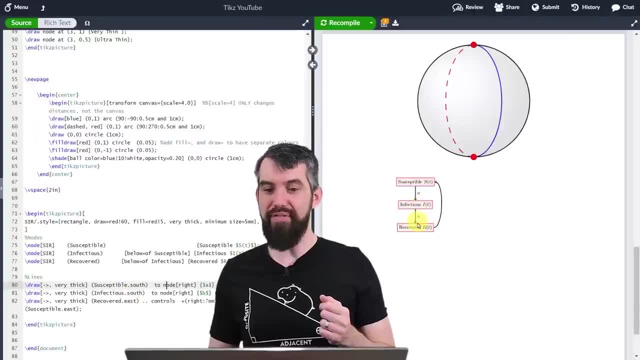 Likewise for going from B. It's going from the south of Infectious to the north of Refectors. So there it is InfectiousSouth to RecoveredNorth, and it to its right. it writes B. Final thing- and this is kind of cool, I have this sort of 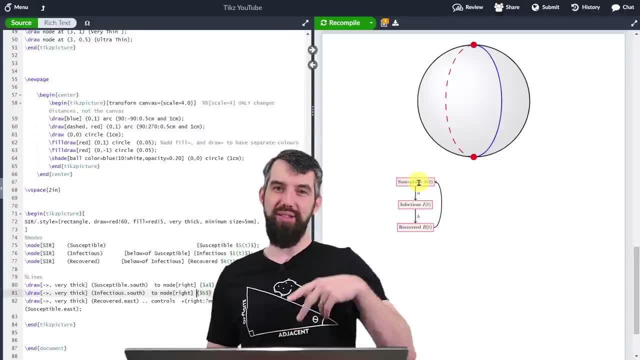 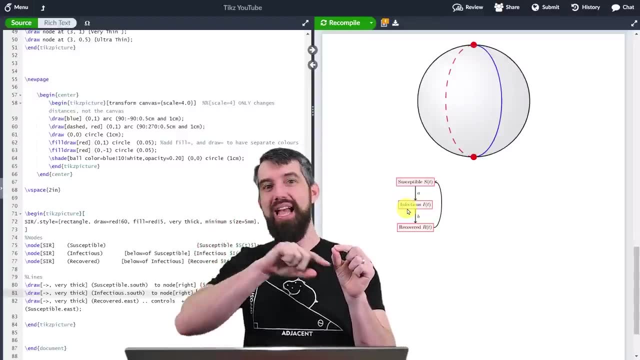 Twisted arrow here, kind of curvy arrow. You can make any Bezier curve that you so wish. A Bezier curve is like you draw a bunch of different points and it nicely Smoothly tries to draw a curve in between those. Basically You do Is you specify the beginning and the end, but also control points in the middle. that 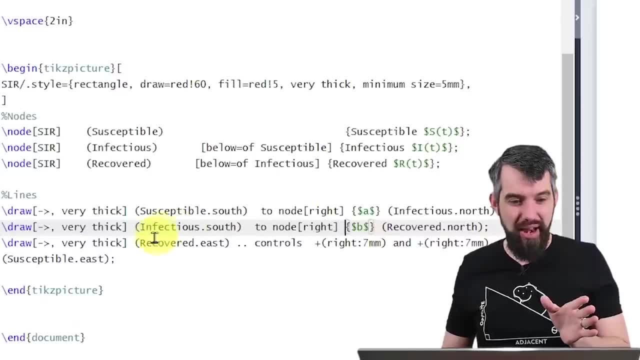 Specify how sort of curvy it's going to be. so this is what I've done. I've started from the east side of recovered and going to the east side of susceptible, so from down here over to there. But I add these control points where I say I want to go right seven millimeters, up to again a right of seven millimeters. 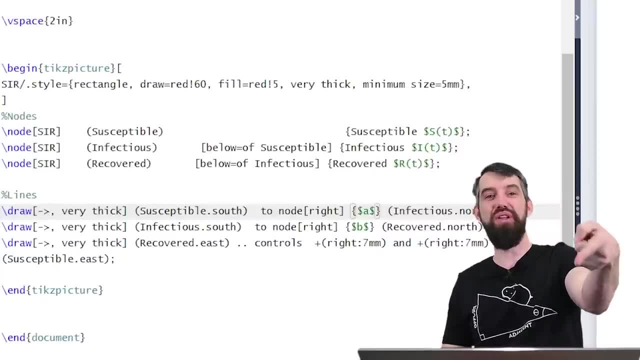 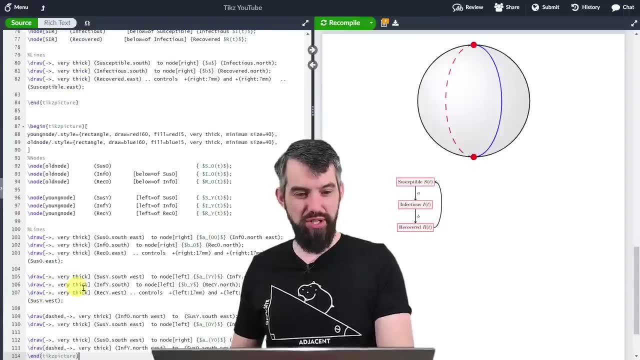 So it's kind of like these points They're sticking out here and it forces this curve that goes out this way. So if you ever need to tweak stuff, you tweak stuff with these control points. I'm going to go and show you a more complicated version that I've typed up, very similar to what we just talked about here. 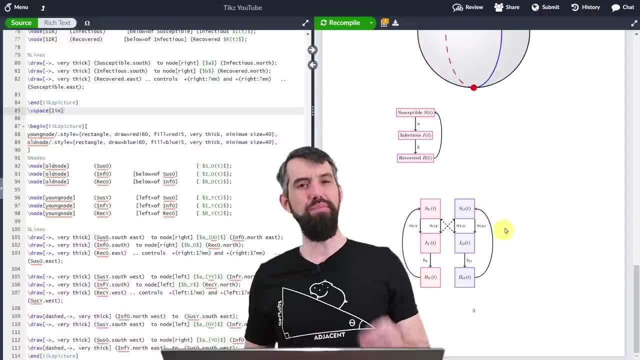 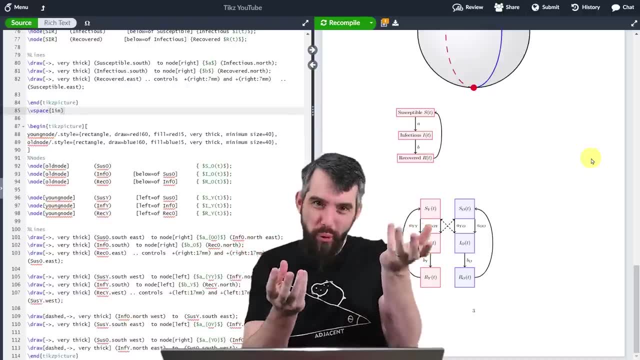 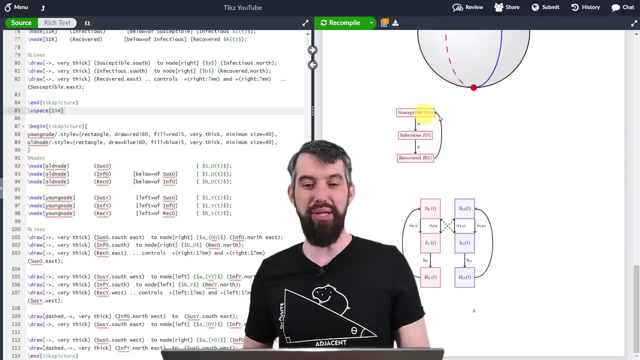 Let's go and give it some space. This is just a more complicated version of the model. for example, one property You might notice if you're talking about pandemics is that people split between older people and younger people, and the different properties of the pandemic affect them in different ways, and so maybe I want us to split this s of si, our model, into an. 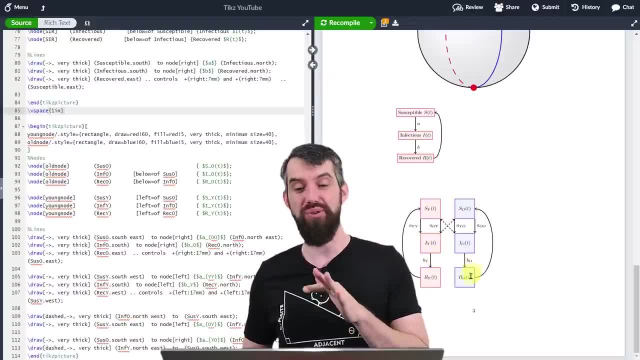 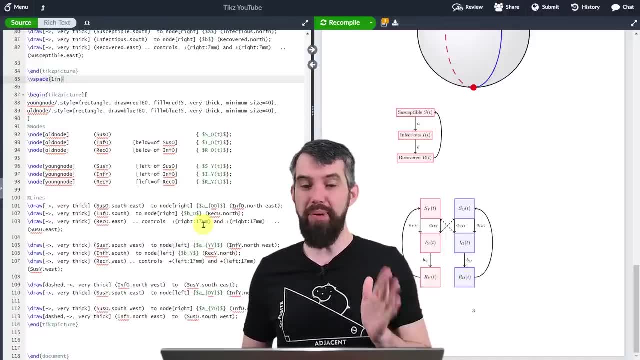 S young, I young are young and an S old, I old and are old. That's a that came off the tongue weird, but nevertheless It's just a more complicated diagram now. It's a big piece of code, but I want to illustrate just a couple things about this big piece of code. 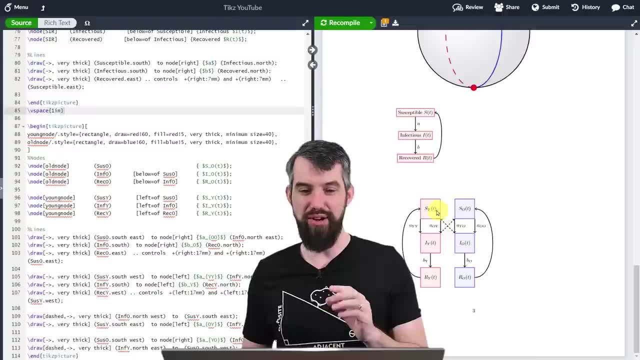 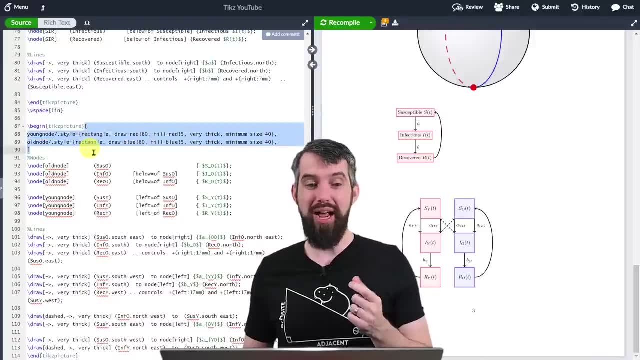 So the first is I noticed that I have two different styles that I wanted to do. I've got these red boxes for the young people, these blue boxes for the old people, So we're previously inside of the square brackets. I just specified one different style, which I'd called si R. now I have a. 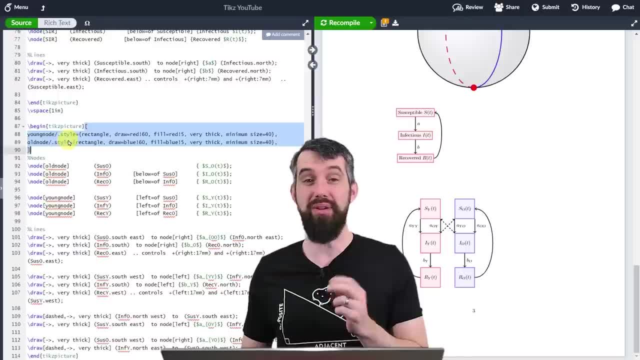 Young node and an old node and I specify those styles to be well similar, But the young ones have reds everywhere and the old ones have blue. So that's how I get these two different styles and you'll see when I create the nodes down here. I have some nodes that are all have the style of old node, some which are gonna have the style of a young node. 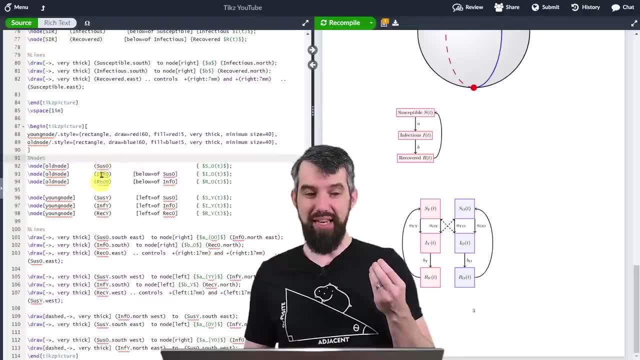 Other than that, the basic ideas are the exact same. I specify names for all of these locations, I give their values, the things that are actually displayed inside of the square brackets, and then I just relatively refer to them left of Sus old or below of sus old. 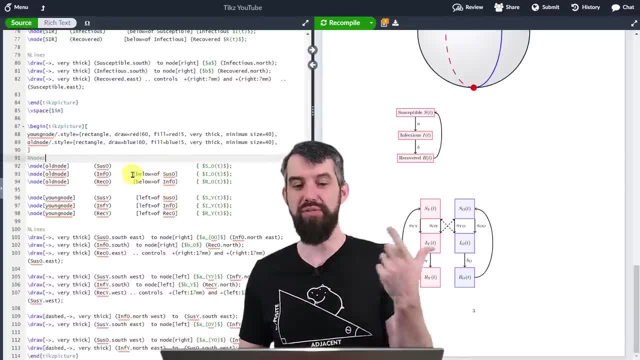 It's just a sort of a reference to the locations of all of these different objects. I fill in all these different arrows and you can get a more complicated description like this. All right, that brings me to the end of this little introduction on Tixie. 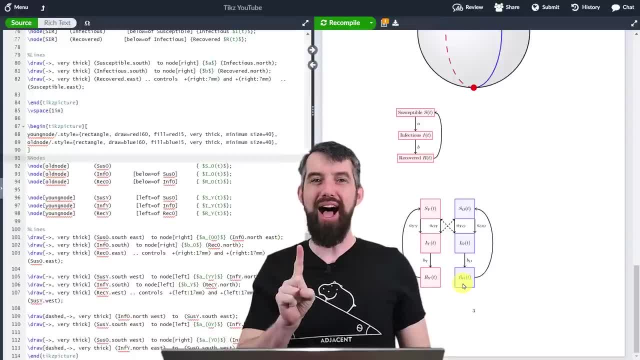 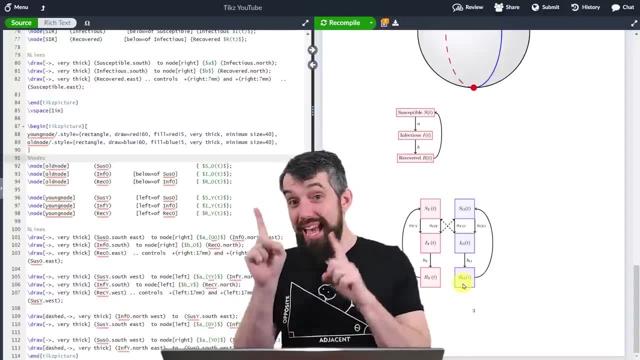 I want to be clear about just a few different points. First of all, I have only scratched the surface of what you were able to do with Tixie. There's a whole bunch more. in particular, in the next Video I want to show actual graphing. 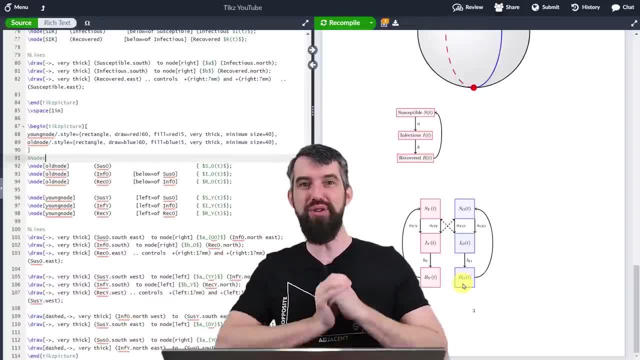 We're gonna dive into the PGF plots a little bit more, So I want to show you how you can make all of your plots in terms of Tixie, as well as, as well as sort of the more diagrams that we've been seen in this video.